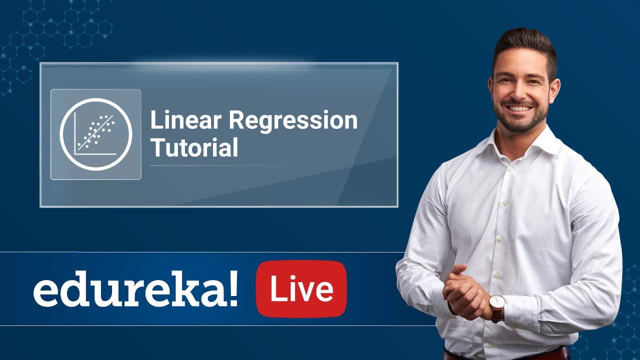 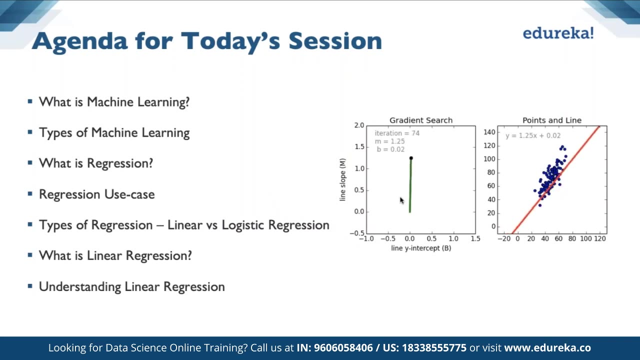 Welcome you all to our session by Edureka, and our session is on a topic: linear regression. Our today's agenda is we have to learn about what is machine learning, type of machine learning. What is regression, use case of regression, type of regression, like linear versus logistic. 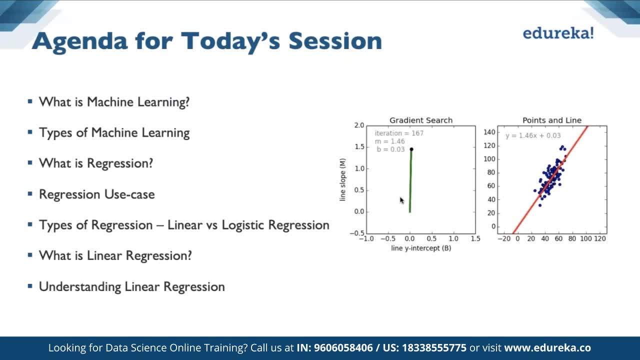 What is linear regression? understand the linear regression. So this is our topic for today, guys. So let's pick it. The very first thing that come into picture is: what is machine learning? means It's very much trending, is a very much buzzword. machine learning, 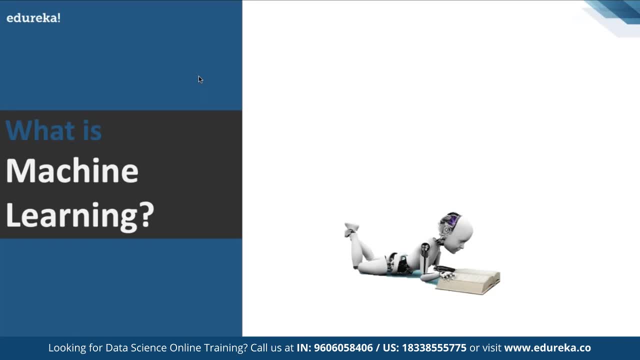 machine learning. What is that actually, guys? machine learning is a quite buzz, because machine learning is. you can say that training the machine is making our machine to learn to do a specific thing. Then we have to make our machine to learn to do a specific thing. 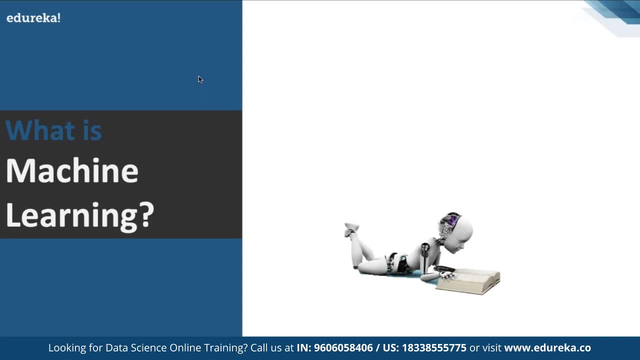 So why so? so that, going forward, if we have to achieve some functionality, instead of we doing the thing, machine do the things for us. Okay, you don't be doing the things, machine do the things for us. That's where the machine learning come into picture. 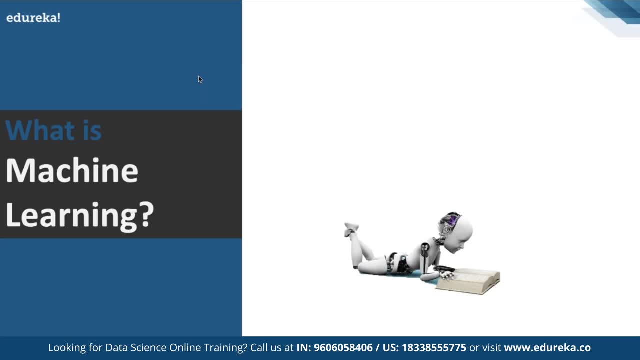 So you can say that machine learning is more or less refer as training your machine to do a one kind of a task, so that next time when the task come into picture you can say that machine learning is more or less refer into picture, that machine perform it automatically. 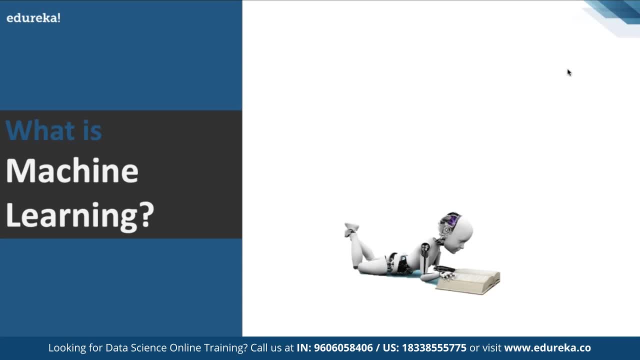 without the human internet. So then the machine got trained. So what happened actually, machine next time able to perform the task automatically. So machine is learning is a type of artificial intelligence that provide computer with ability to learn without explicitly programmed. machine learning focus on the development of a computer programs. 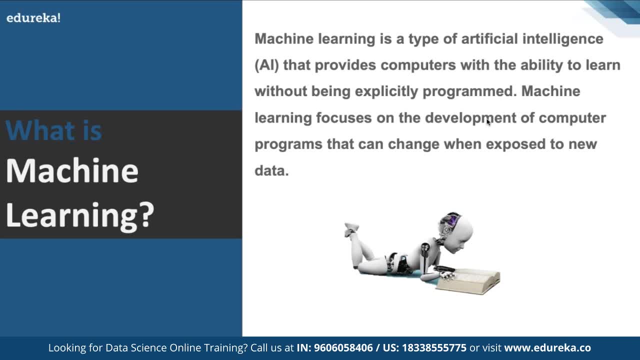 that can exchange when exposed to the data means I said no like and in the machine learning know. the point is like that machine learning is something where we have to keep on enhancing the thing. machine learning in working away that very enhance itself according to data and they have something called as a self-learning model also. 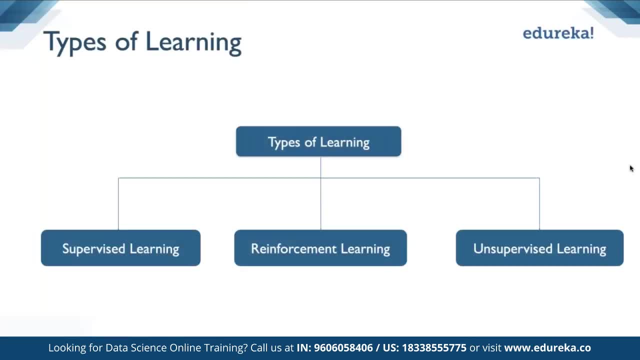 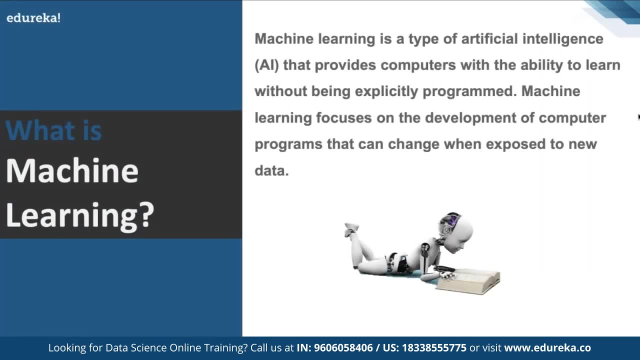 So and to the three things: one is called as AI, One is called as your machine learning, one is called in a deep learning. What is that actually a bigger box? If I say one bigger box, the outer, and a bigger box is that AI, machine learning, is a part. 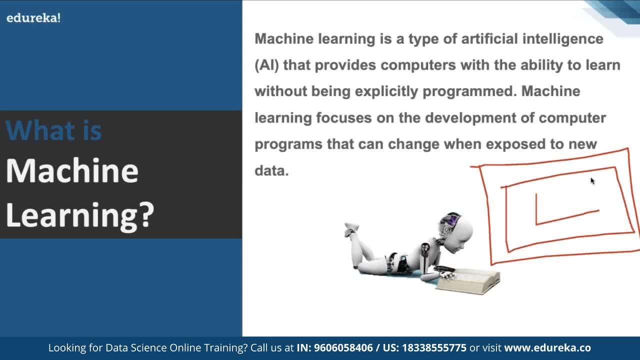 of AI and deep learning is a part of machine learning, with the outer one is a AI, The inner one is a ml and your inner one is a machine, The outer one is a DL- deep learning. So AI have all these things like machine learning, deep learning. 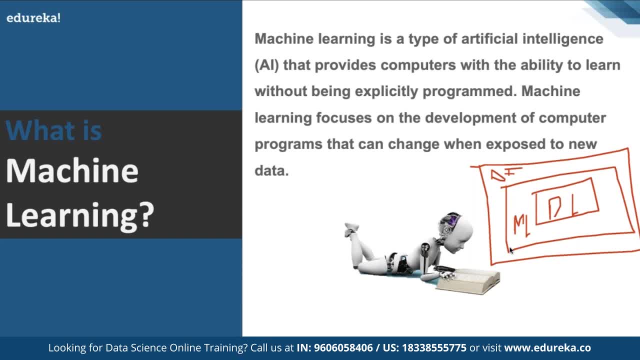 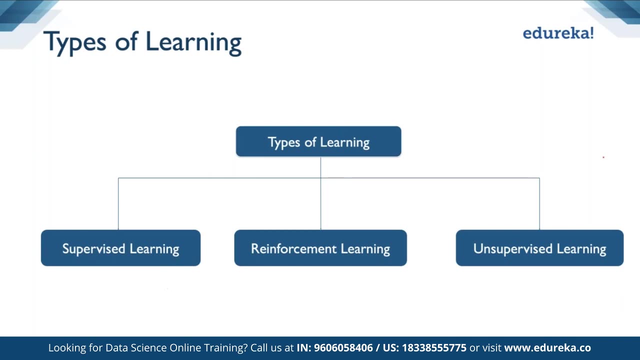 will not part of a AI and a deep learning in the part of a MP. That's how these two things are placed into one stack. Now next thing again, machine learning is of multiple type: supervised learning, unsupervised learning and reinforcement learning is a very common interview question. 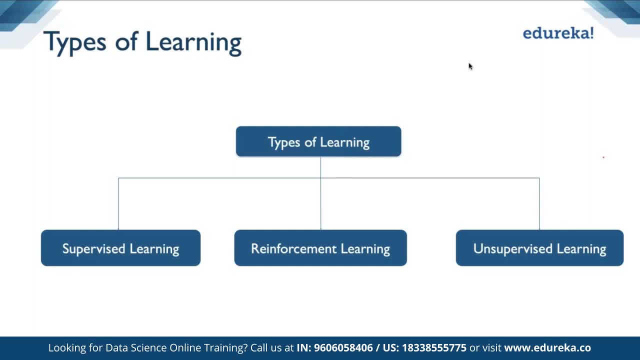 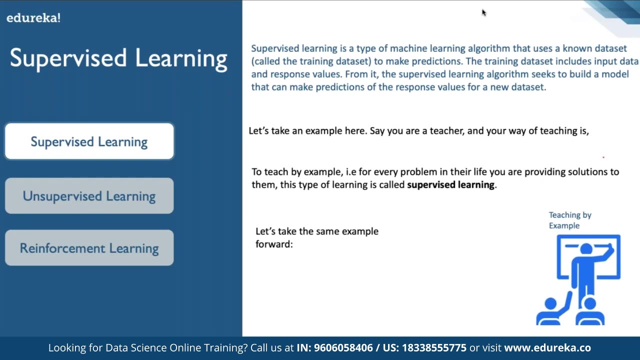 and then, for sure, ask questions like that, 100% ask question on the interview. Now, what is supervised learning? supervised learning is a kind of a learning where we are training our machine for each and everything is and everything is like whenever we get any set of a data. 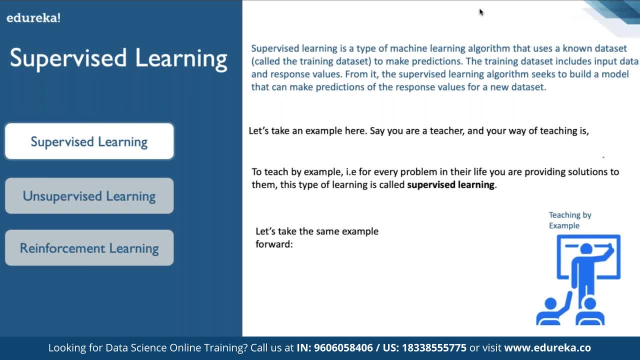 We trained our machine to tell that: okay, this is this, this is this. suppose we have to have a thousand of images Now, first of all, before, like I have a 10,000 image for 10,000 image, What I'll do is very first time. 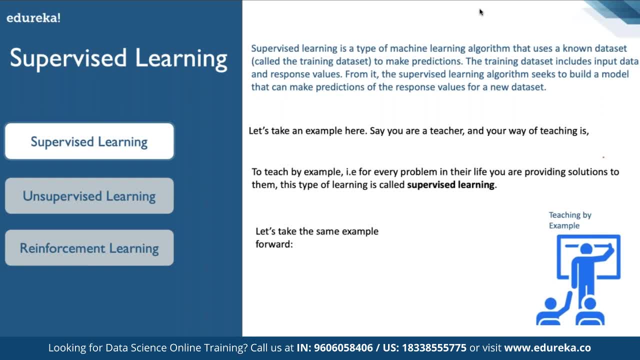 I trained my machine for all those 10,000 image manually. You have to feed your machine manually, which you will tell the machine that, okay, This is car, This is bus, This is bike. like that way, We have to keep on training our machine. 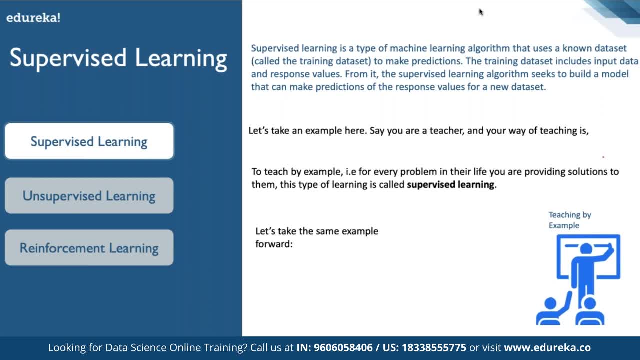 First of all, I mean this is our job: to train now, Once your machine got trained- like you are responsible For training the machine. and once you trained your machine properly, then after that, suppose you train a machine for 10,000 records, although we try on train for very huge amount of a data set. 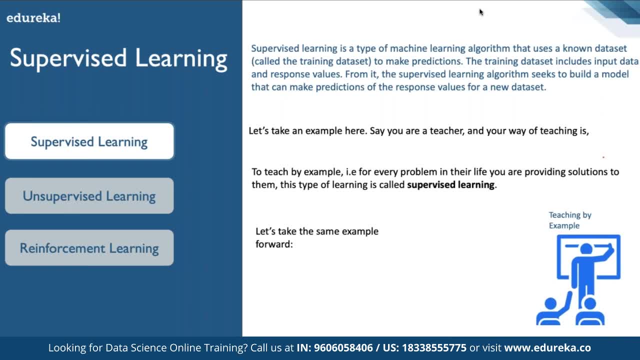 But as example, suppose I train a machine for 10,000 records now after that, if I pass, show I have password image, then machine can identify that what this image is all about. But that is supervised learning. We have supervised our machine to trained for something. 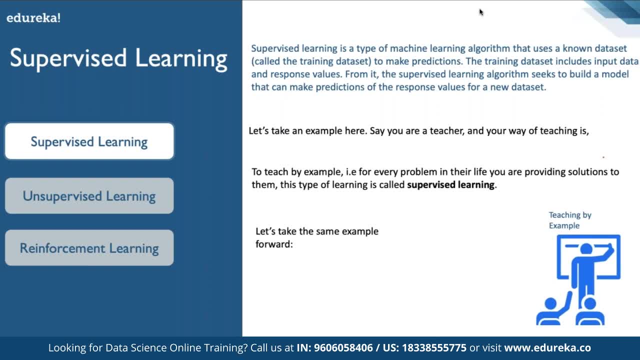 We are. we have trained the machine And, on the base of that machine, predict. and that's what is happening, guys, 95% of the case in the market right now in IT are supervised learning. Believe me or not, There's nothing called automated process- 95% thing. 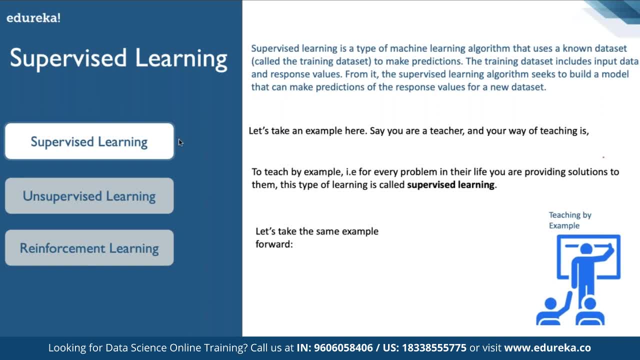 in a market is supervised learning, where we are training our machine and after that machine behave or answer in that particular manner. So supervised learning is a type of a machine learning algorithm that use the that used, known as data set, called training, to predict. The training data set include the input data. 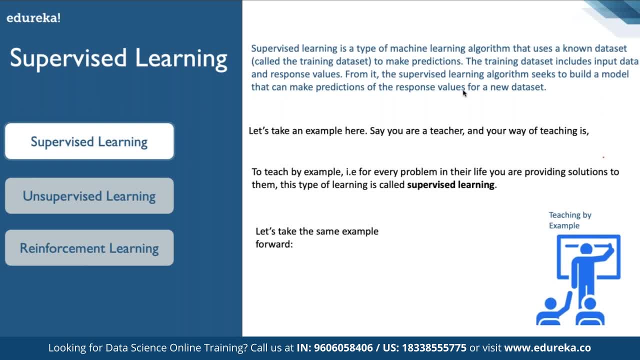 and the response value for it. supervised learning algorithm seeks to be a model that can predict, prediction of the response value of a new data set. Let's take example here. say you to your teacher: So, teacher, and you are teaching your, you are. so your way of teaching is to teach by example. 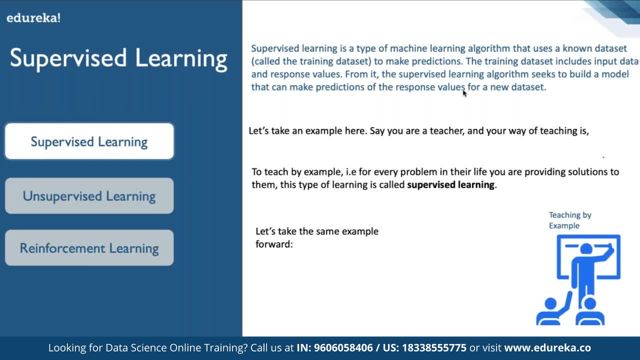 that is for problem in your life. You are providing a solution to them. These are way called supervised learning, means your teacher is telling you the problem statement also and teacher is telling the answer for that problem statement also, because they are telling that how to approach that, how to answer that. 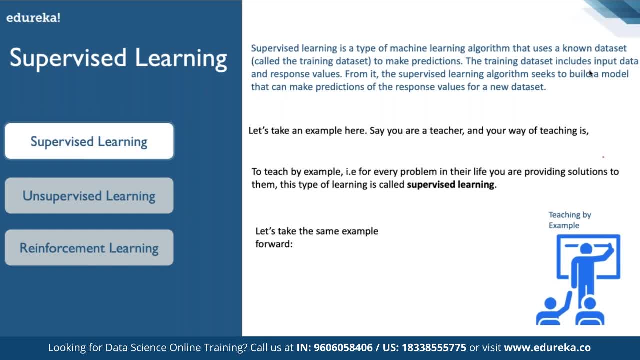 and they have did like five, six questions like that. Suppose, in a junior classes, when we go for a mathematics or a physics class, our teachers perform some two, three examples for us. right after that, the next example we are able to do because we know that this should be the question. 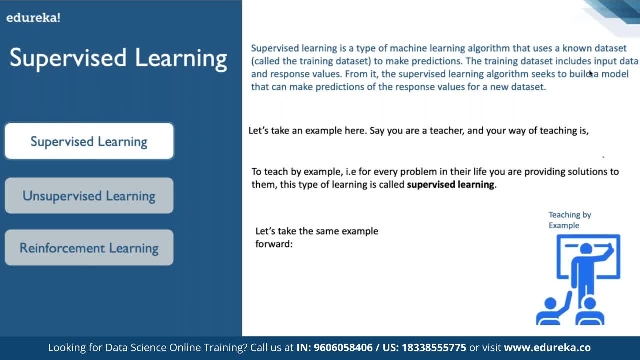 and that this question, have this answer. Now there's a way to get that answer. and now, once we know that, So we are trained for answering that question. and once we are, guys, trained for answering that question, There comes a point that you have trained a machine. 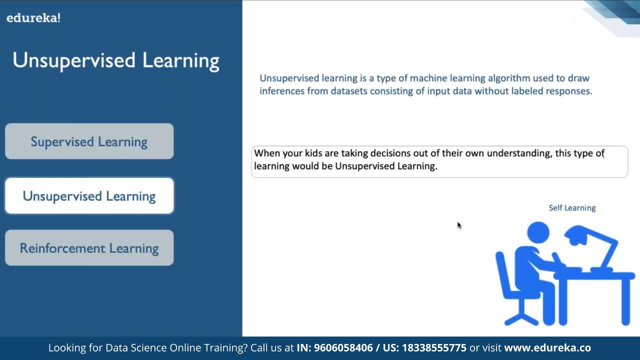 in a supervised manner. The next is unsupervised learning. What is unsupervised learning? unsupervised learning is a type of machine learning algorithm used to draw inference and data set consists of data without labeling response. So unsupervised learning is one thing. when your kids are taking a decision. 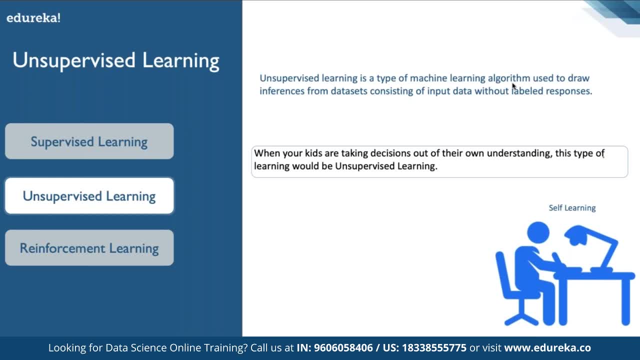 of their own understanding. this type of learning by would be called unsupervised learning. Everybody say our bot is super trained, it learn by itself. Those are both unsupervised learning, where they understand the things by itself, without training. I tell you guys right now: 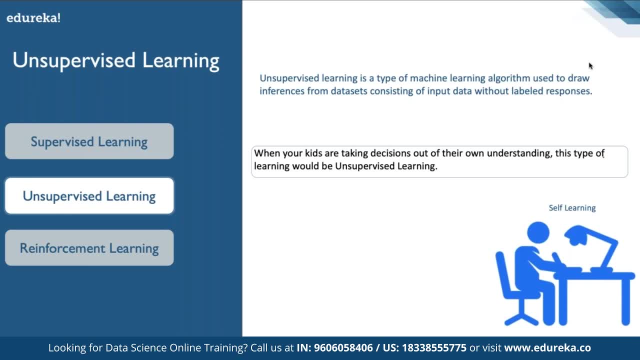 No machine is there that work on hundred percent unsupervised learning means it automatically learn from by itself. means you give some data, it understand that data and behave on that. I'll tell you one example. around two years back, Microsoft have launched one row or say one chatbot by the name of pay. 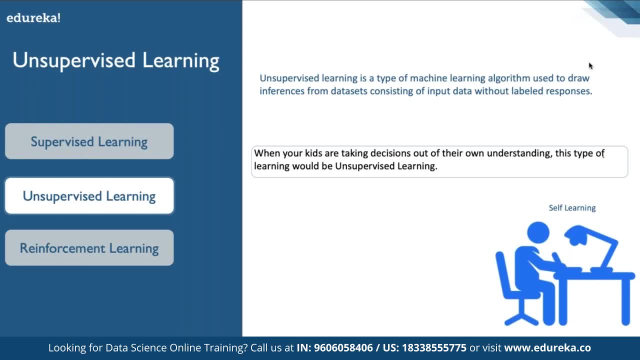 I'm not sure how many have heard that story. Pay day was a one, say, chatbot. What that they do is for a taino. They just have to feed them with a Twitter feed. Say, we can feed the table Twitter feed. and they was kept to learn from the Twitter. 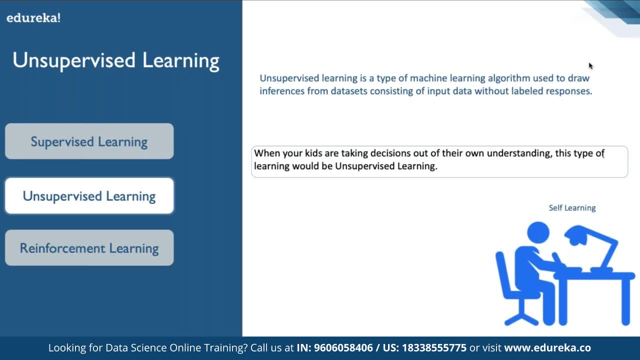 So you tweet something, they learn that Twitter feed and try to create the response for itself. Now, what the people did with that. actually, people played with that very badly and in just two hours means just two hours. Read the story of that: Microsoft a in just two hours. 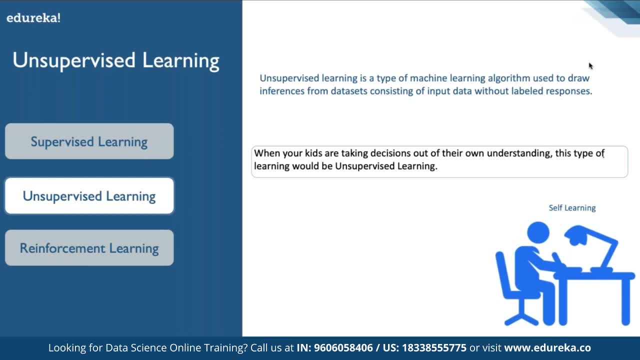 that project got shut down. Why? what the people it is. people start training that chatbot, Chatbot with all the bullshit things, all the bullshit. like people start training the robot by the day. Okay, I'm the master of the world, I'm going to kill the world like that with that. all way, people start training. 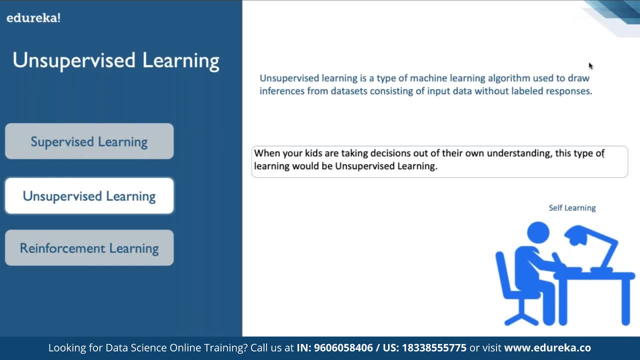 and after that, when anybody and asking the robot, they are answering that in a very bad manner. So ultimately, what happened? the Microsoft have to shut down their project in two hours because that way is unsupervised kind of learning and the unsupervised learning it become difficult. 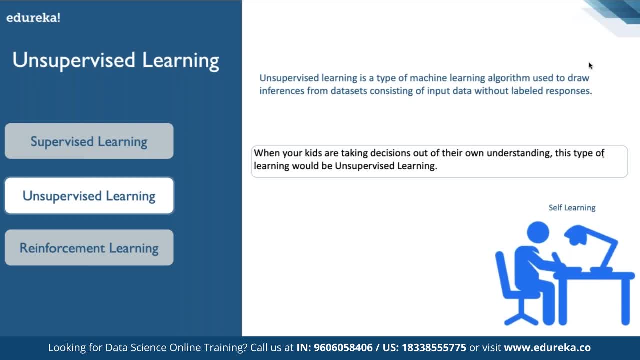 for them to control that. so, guys, these days We don't have do of unsupervised learning in any domain. You go all the everybody say that our robot is, our bodies doing this, our machine learning is doing this, We want to provide like that way. 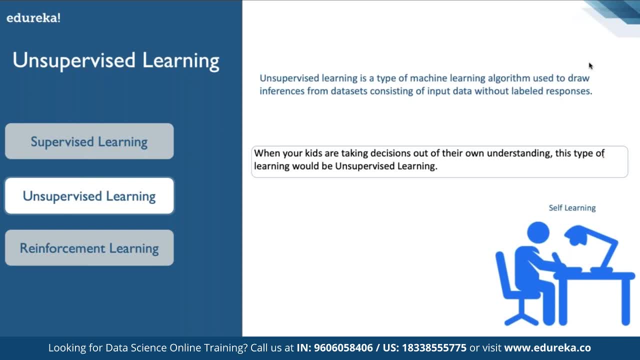 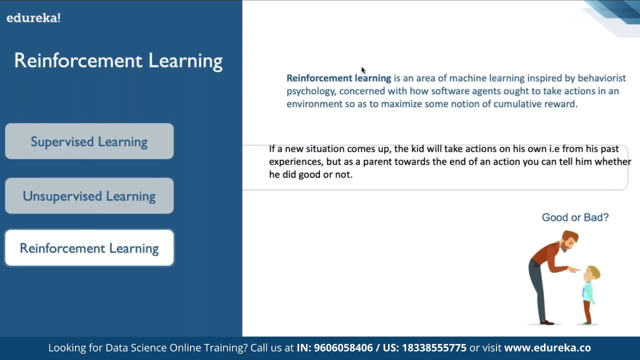 but I tell you one thing Generally is not like that And guys. then other thing is called reinforcement learning. reinforcement Learning is that learning from it mistake is like improving itself from it mistake, Like what happened, like first of all we train the machine. 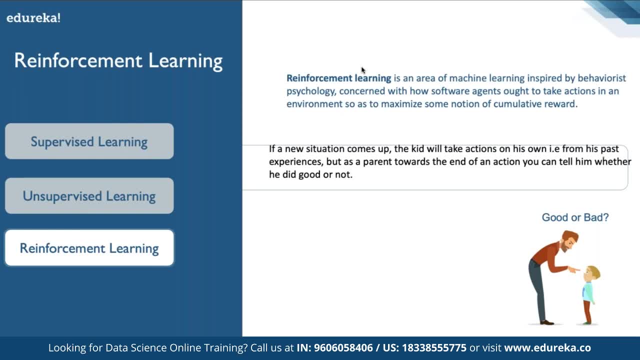 Okay, we train the machine for few entities or intent, or say two different kind of responses. Now, after that, what happened when we actually trained our machine for few different responses, know, After some time, machine, now machine have to start learning of its own. Okay, machine start learning of its own. 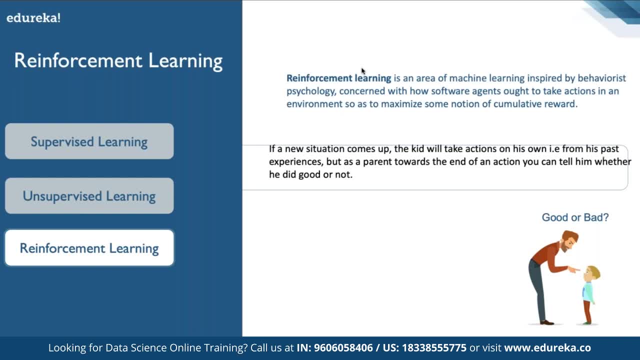 in that case, what happened? machine, try to repeat the same thing, the one you said after that. you score them. you, as a user, score them in the scoring. you will tell that. okay, This is the correct response. This is a bad response. machine try to learn the things of itself. 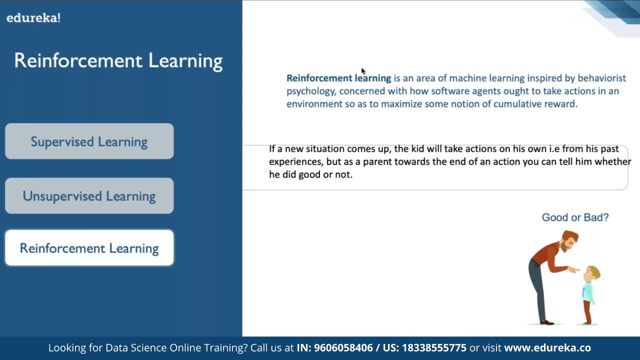 Okay means first you train it, Then machine get a lot of questions when a machine try to use those questions. So machine try to use those questions and machine try to train itself and on the base of the score You will tell the machine that this is right. 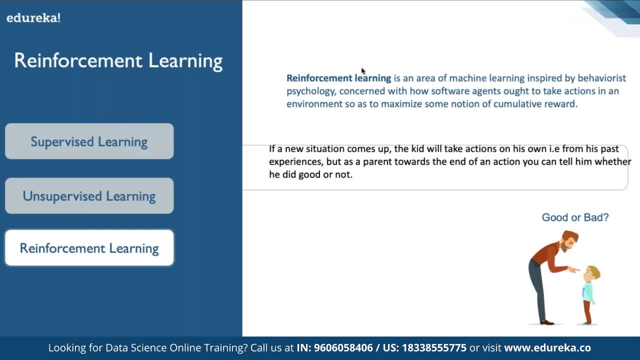 This is wrong and whatever. tell the machine: This is right machine, Try to learn, go in that direction and try to increase its performance. in short, You can say that, as a child, when we do something right, our parents say That, okay, as this is right. 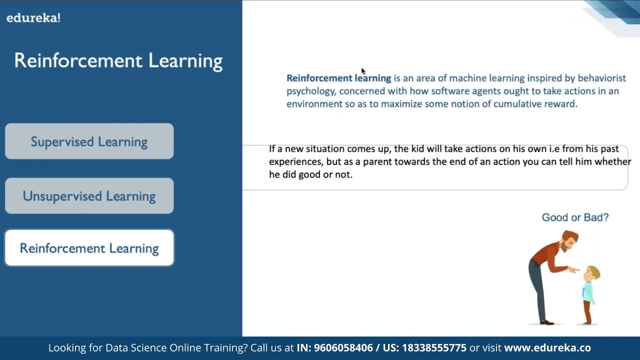 So we know that this is the right thing, and we start doing that thing in more numbers, many times more, like that, Whereas if our parents called us say no, this is not right thing, Then we know that this is not the right thing in that case. 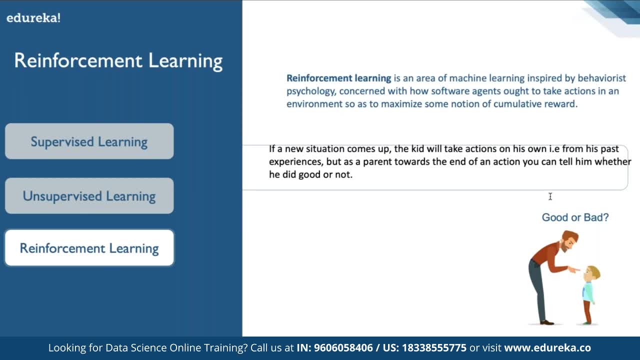 What happened. We know we should not go in this direction. So, guys, this is called reinforcement learning. So reinforcement learning is an area of machine learning inspired by the behaviors or psychologists concerned with the how software agent taught to take action in an environment. So to maximize some notation of a cumulative rewards. 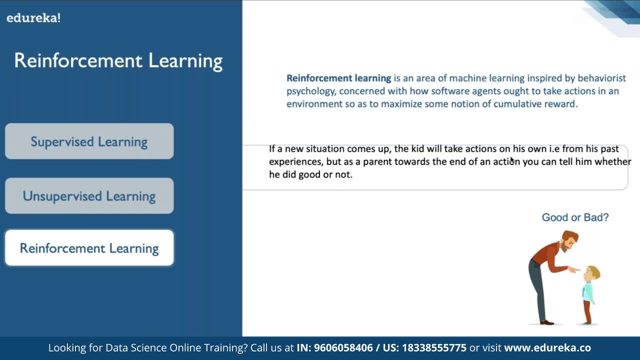 if a situation come up, a kid will take action of its own. you, from his part, experience, past experience. but a parent, toward the end of action, You can tell him whether he did good or not. in short, like we tell the machine on the base of the confidence score. 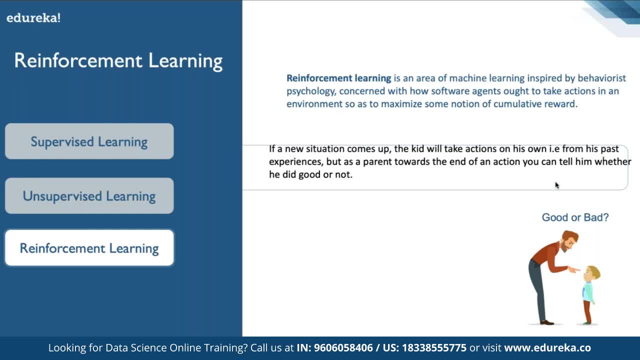 that you are doing a right or wrong. And when we tell those things to machine, machine know that they have to start going this particular direction. That is what is called reinforcement learning. So, guys, these are the three major, in which one, in one case, you are taking care of each. 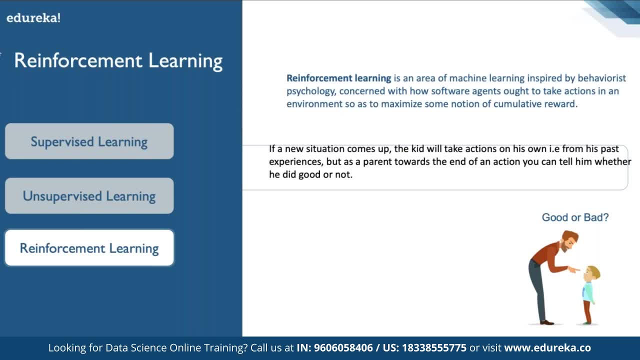 and every data for a best response. This, the first supervised learning, is the one that gives the best response. then unsupervised, something that don't give the best response, and the reinforcement is also give us a best response because it keep on training the machine of its own. 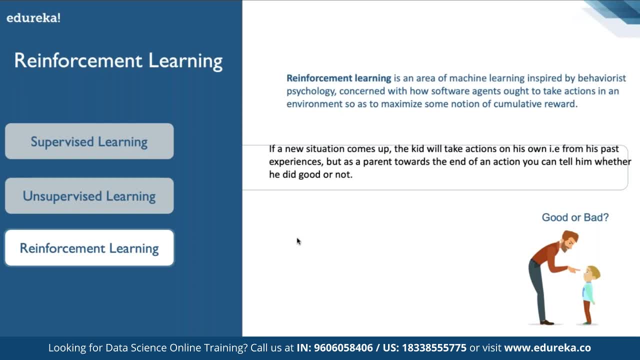 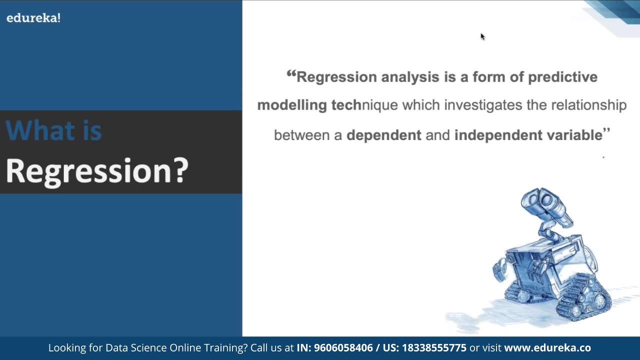 on the basis of a different result or on the basis of our, say, responses. Okay, Now let me talk about next thing, called regression. What is regression now? regression is an analysis. So, basically, what is regression? regression analysis is a form of predictive modeling. 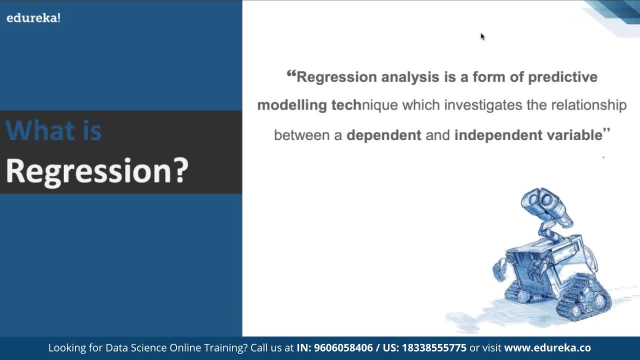 technique which investigate the relationship between the dependent and the independent variable. Regression is something we are- one dependent variable and one independent variable. We figure out how XV does I trade over the things in our own fashion and figure out what should be the best response for that, as example. 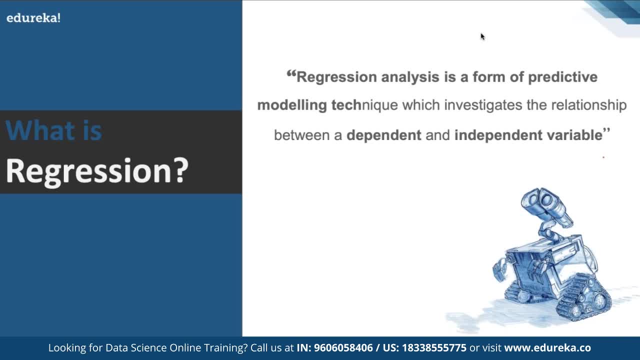 I want to predict that how much sale is going to happen next year or next month. So I have the previous sale figure like what product sold more at what time of the month. So ultimately, as example, like it's a grocery store the very first week of a month, 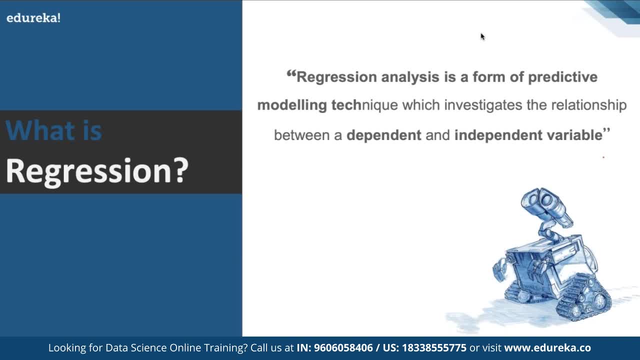 We notice that people are buying more staples. people are buying more, your say, in terms of like oil And whatever the floor, whatever they need in a daily basis. and during the mid of the month We see that people are buying some occasional stuff and at the end of the month the sale decreases. 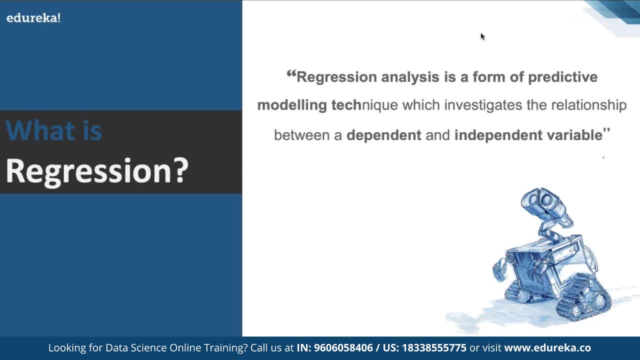 because people are running out of the their budgets. So we have to forecast that, what exactly we should plan. How much inventory should I keep for a month and what kind of inventory should I keep for a month so that at the end of the day, week having our best output? 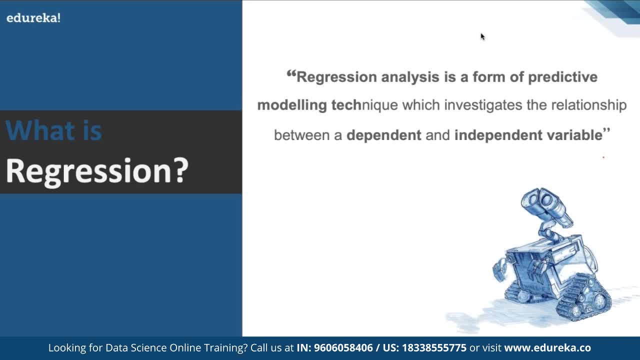 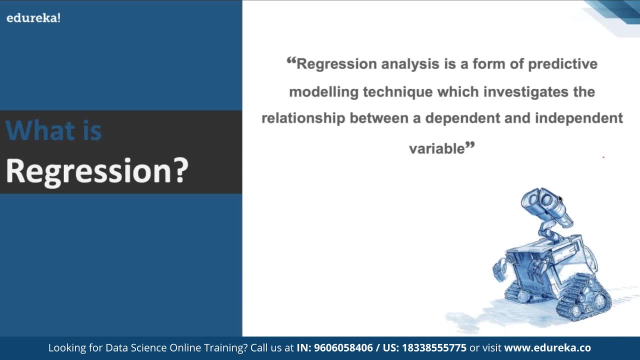 and best result. So that is what we have: one dependent variable, one independent variable or other way around. I want to figure out that tomorrow the match is going to happen or not. in that scenario, Again, I have to check that say, what kind of weather is this, or it's a public holiday? 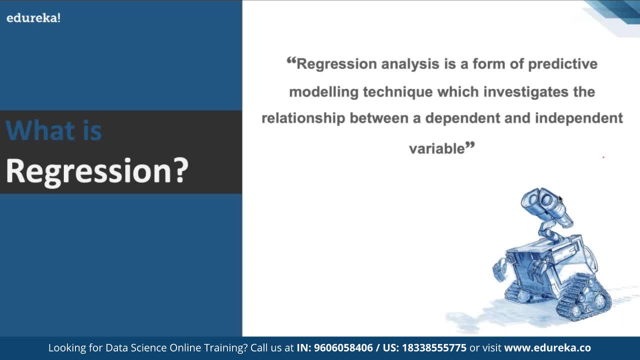 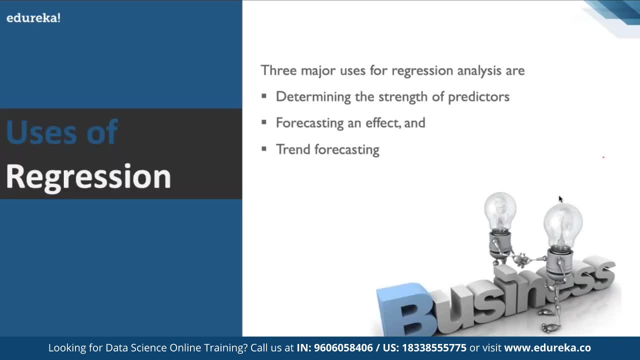 or not, How much audience I can expect for a match, so that also we can check. we have one dependent and one independent variable. regression is something you, I trade over something and get the output. So the three major use of regression list I told you know one is called determining the strength. 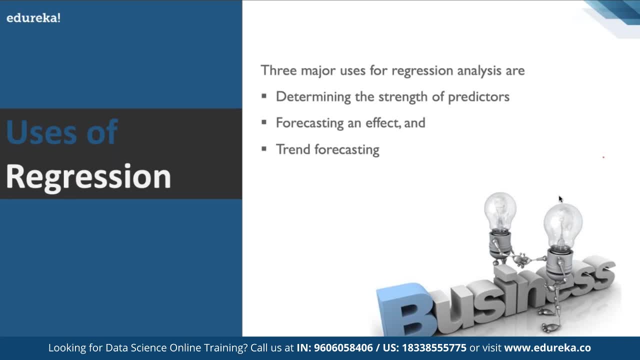 of predictors, forecasting and effect and trend forecasting. We'll tell that what is going to happen next. So, guys, this is a very, very important part of a business. any business that you see around want to know that how their business is going to be happen in next month, because accordingly, they will plan accordingly. 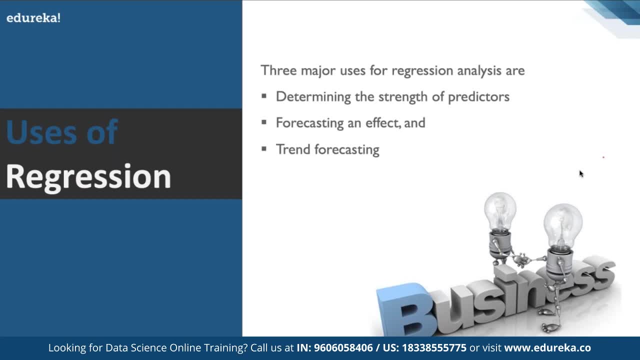 They will decide that, how, how much workforce they increase, how much time they dedicate. all these things they define or decide from basically their forecasting model or from their regressions. So regressions are very commonly used terms in your machine learning guys. Although the multiple will doing it, getting a regression done. 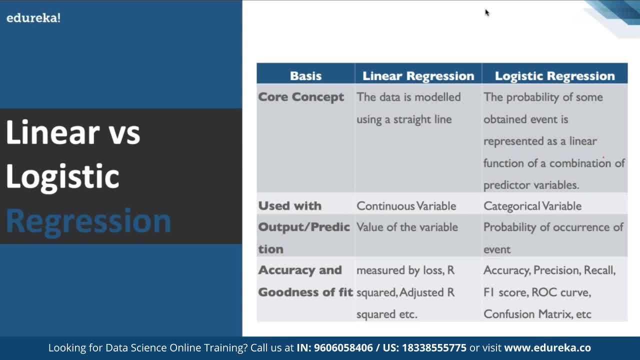 but are two most popular regression You're come are. one is called as a linear, one is called as a logistic. Our focus is on linear for today- for this particular webinar might have been upcoming webinar- We'll talk about logistics also. So linear, linear data is a modeled user straight line. 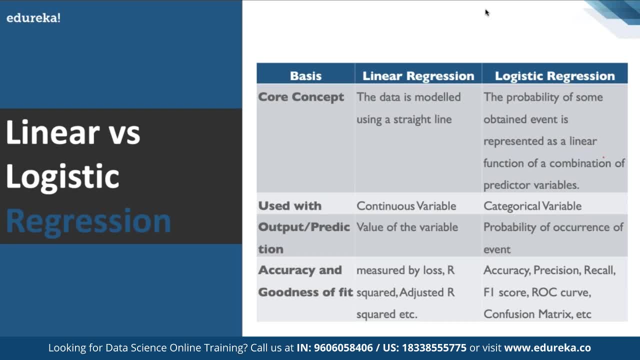 in a linear model We draw a straight line and we find out what all points are near to that state Line, and if they're far from a state line then we'll see how far they are and how we can improve that. that's basically a linear regression. 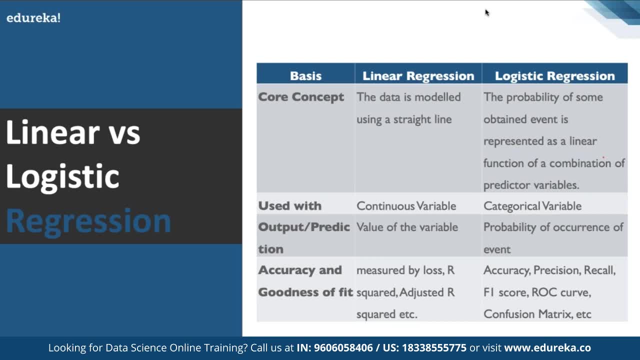 where, in a logistic regression, what we do is the probability of some obtained, is the represent as a linear function of combination of predictor value. So in this case, what happened? we find out that a sum of a total linear regression and divided by the total value, and then we predict that. 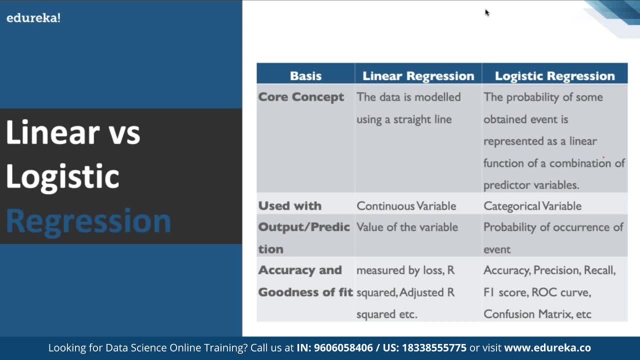 There's a bit different concept. your linear regression use for the continuous variable means have a continuous data, like for this, one hour to first hour. We did this second hour, We did a third of the. we did this so that kind of a continuous data or quarters variable. 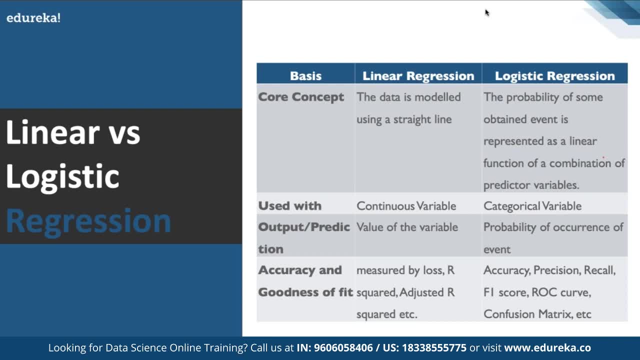 We go for a linear regression and in terms of categorical, categorical means, you divide into the multiple categories and they have one independent, dependent variable. that go for a logistic regression: Output: value of the variable and probability of occurrence. This will give the actual value. This is the probability of that. now, accuracy and goodness of fit. 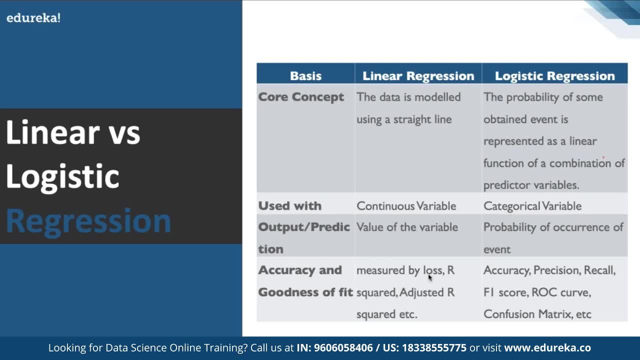 How we can measure the equation. goodness of fit, measure by loss. R squared, adjusted R square. I said no, we draw one straight line and we'll see what points are near to that straight line. If they're far from a straight line, how far they are. 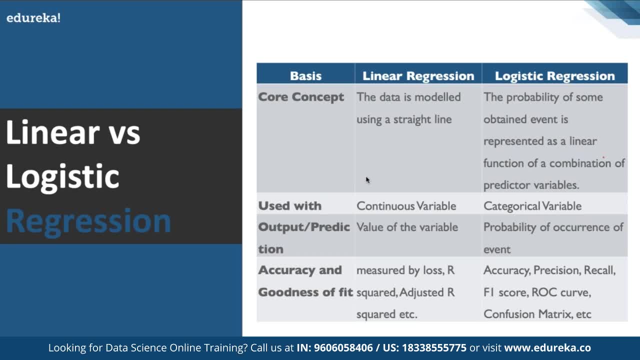 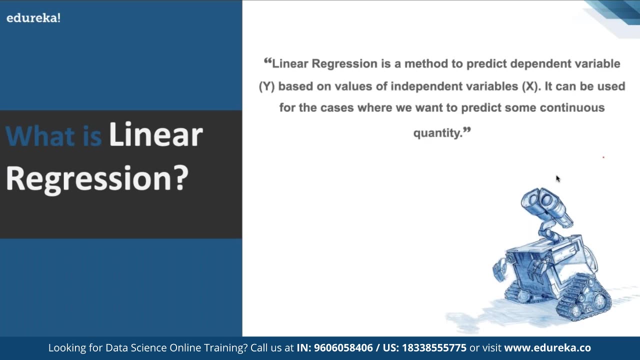 from a straight line In a logistic regression: accuracy, season, recall, FI score, ROC curve, confusion matrix- All these things are used for the accuracy and goodness of it. So then, let's focus now on the linear regression. That's what our topic, linear regression, is a method. 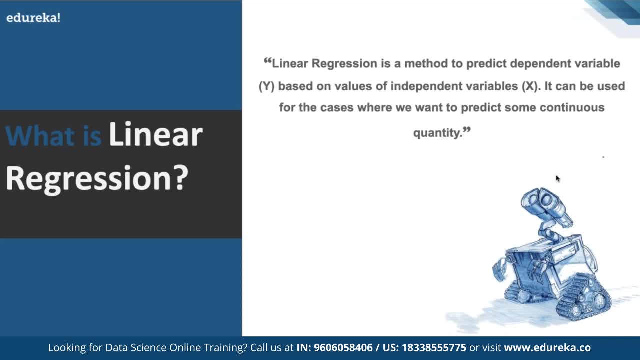 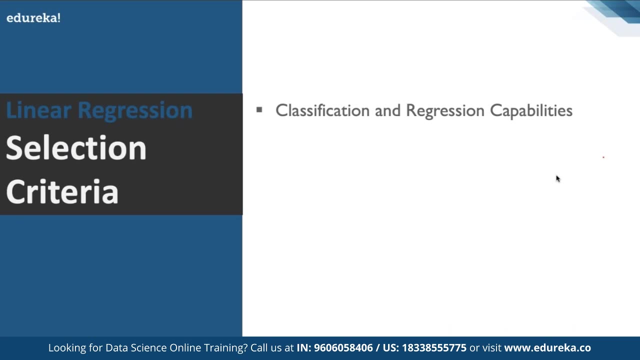 to predict dependent variable Y based on the independent variable X. It can be used for the case where we want to predict some continuous quantity, as example. So what are the selection criteria that we should go for? linear regression, classification, regression capability, data quality, conceptual concept complexity. 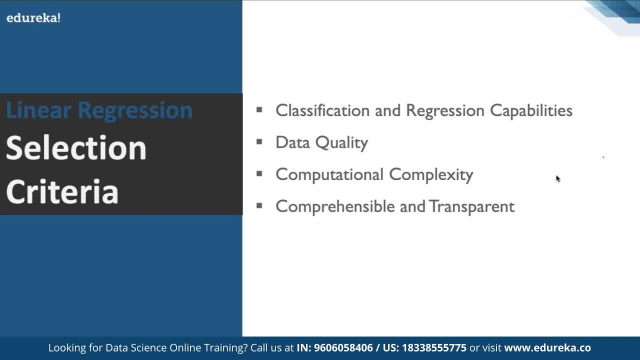 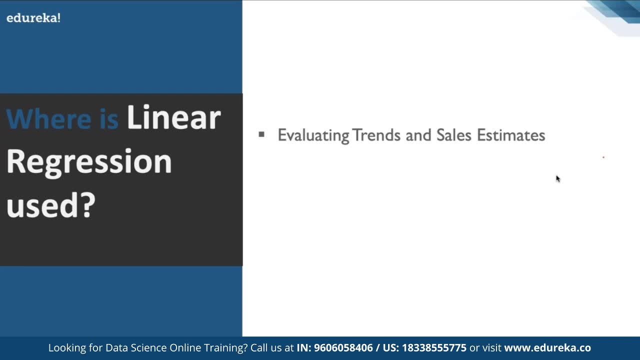 and comprehensive and transparent. These are some of the selection criteria. These are some qualities of a linear regression. Now, where the linear regression used evaluating the trend and a sale estimate means I would trend out or estimate that how much sale is going to happen this month. 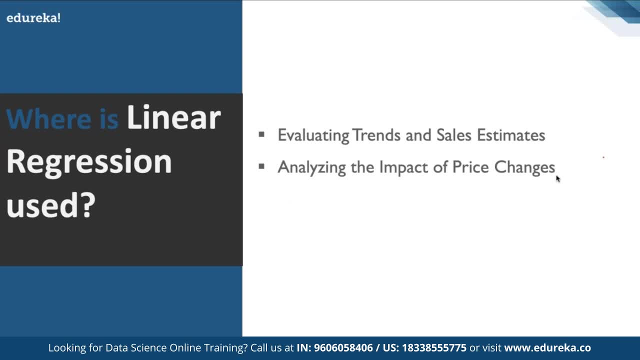 Analyze the predictor price. I want to check out. my company want to know that if we increase the price of this particular product, how exactly the sale going to be affected. or we decrease the price of this particular product, How the sale going to be affected. so that kind. 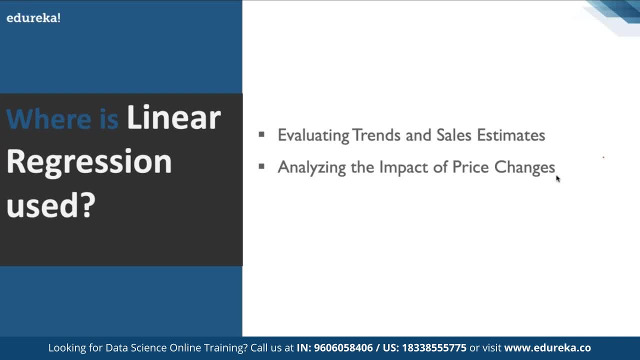 of a trend you take out from the linear regression. again, assessment of a risk for financial service and insurance domain means I want to figure out that. what age group is a? what happened? insurance company, insurance companies- I really have to settle their claims right now. if a person who is young in age they prefer, that day by more policy. Why so? because they know that they are the person. if they claim. also they click. the chances of claiming them is less as compared to a person who is of old age. a person who is of old age will claim very early. They know that they will not even get that much amount. 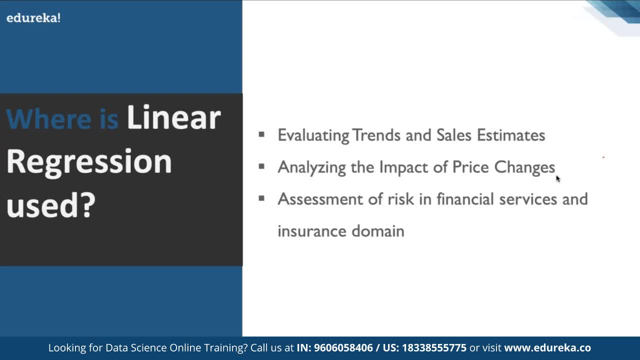 which they have to pay back, as compared to a person who is not very old And the person was not very old. if they actually say Work on the scenario And they actually buy, the interest policy will be the best suited so we can figure out that what exactly we should pick. 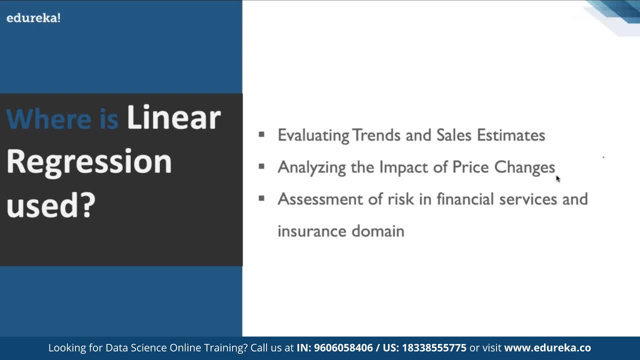 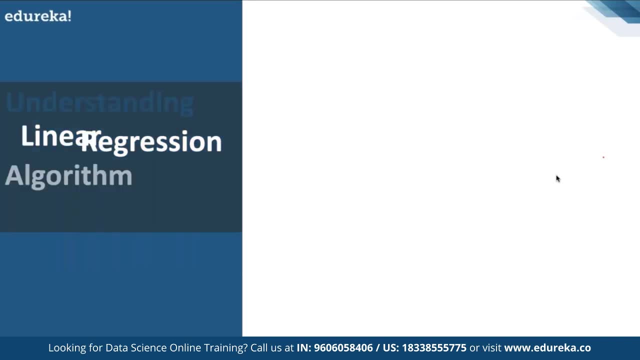 which age category we should pick. that helped me to grow my business better as compared to the. I am not going in a loss for that case. Here we have one independent variable and one dependent variable, And here what exactly happen is your depend upon the criteria. 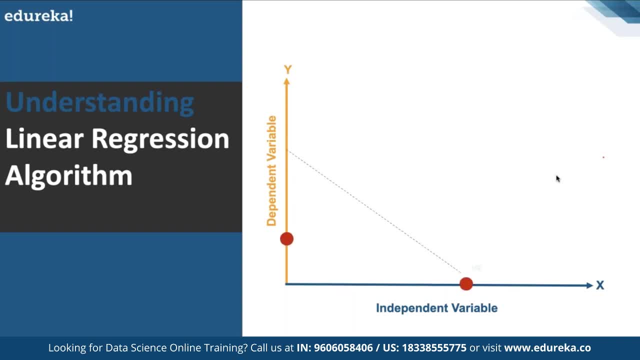 like which variable is increasing means. I say I again show you one thing. Let's see here now, on the X axis We take independent. Y axis, We take dependent variable. We say it: independent variable in Is. and dependent variable also increase means price increase. 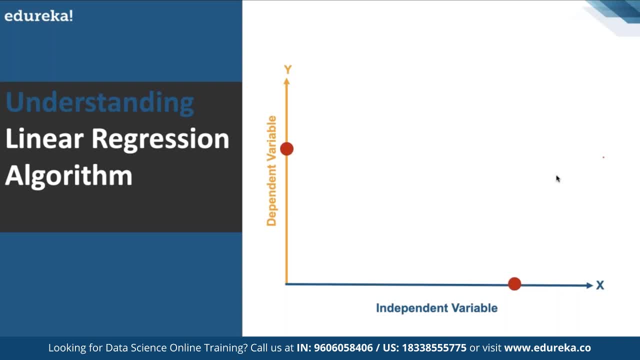 sale also increase. that is basically refer as your positive slow. It is a benefit for us If the dependent variable decrease and independent variable increase, as that dependent variable keep on decreasing means the sale is going down with a price increase. That's a negative slow. 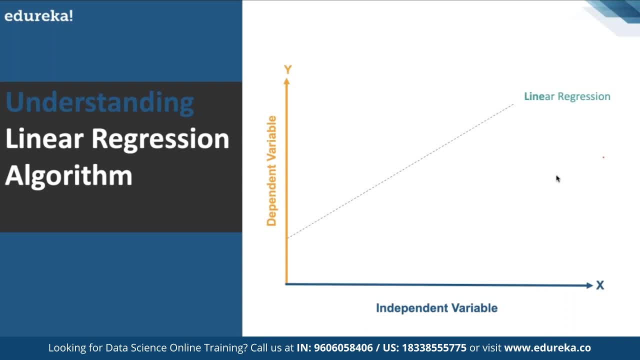 Now we have one straight line, That's a linear regression line. We will tell that, okay, this, this, this should be the probability, and then we take out our observations. So we have one probability that the same should be 60%, and then we have our actual values come up. those value 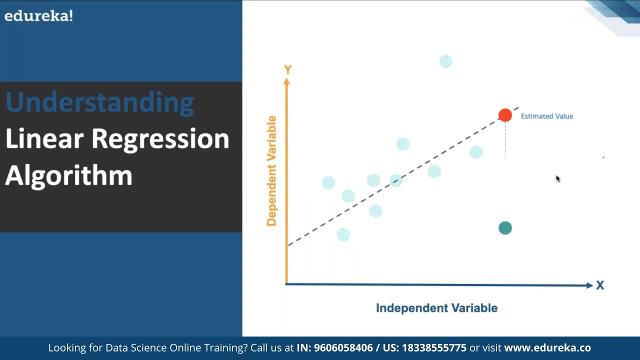 which lie in this particular state line is basically your actual predicted value, and the value which is far from that points are basically reference error as compared that. so according to me, This is my fall under the. under the linear regression model will say: if this much price, increase this much. 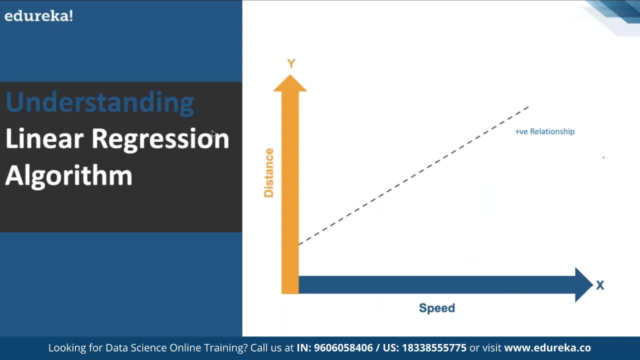 sale will increase or speed versus distance. If we say if a speed of the vehicle will increase, more distance will be covered. I have speed degrees, less isn't will be covered because they're dependent to each other. The formula for calculating your regression is: y is equal. 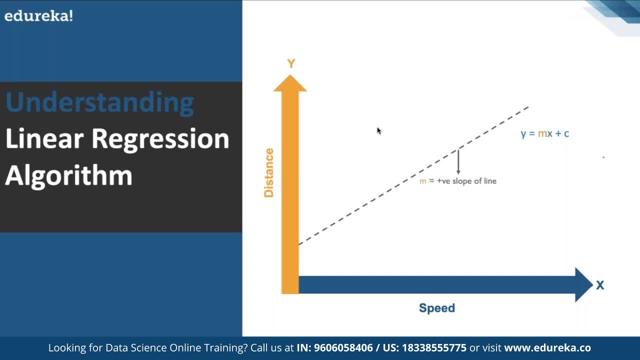 to MX plus C, Where M is a slope of a line, X is an independent variable. and why the dependent variable? and see the intercept, See the intercept where it is drawn. So is a speed increase. time also will increase and the speed increase. 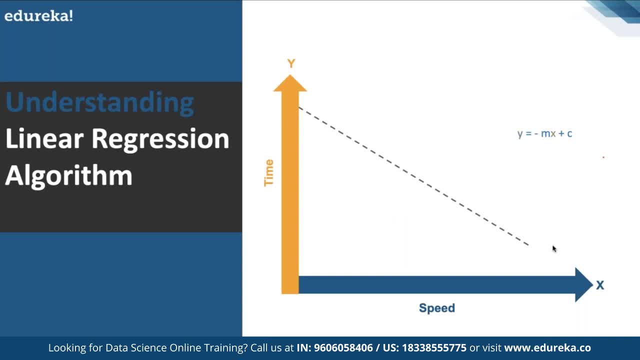 You can create the slope value and on the base of slope value We will calculate what lies near to our slope. So it's a, their y is equal to MX plus C. where why we can calculate? because if you see here, X, Y is the distance traveled. 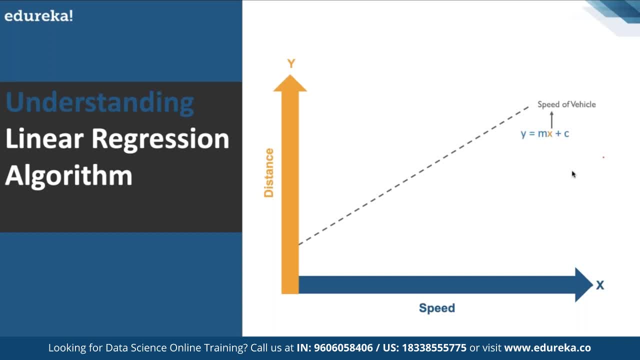 in a fixed duration, X is a speed of variable, M is a slope of a line. Now we can take with the value of C. similarly, in a negative slope, time taken to travel, the fixed distance speed of the vehicle, negative slope line, And there we can talk with the value of C on the other side. 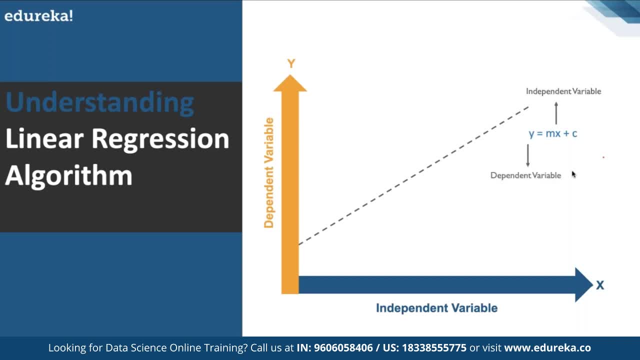 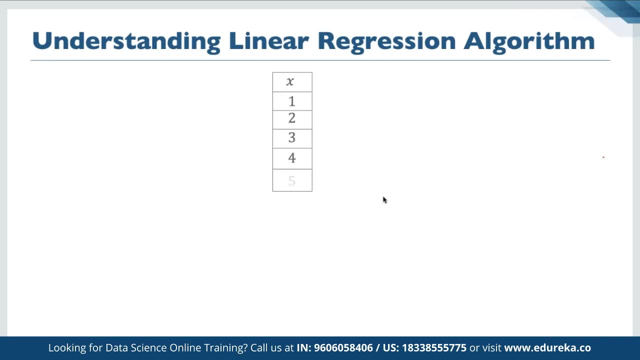 You have positive slope line, We have one dependent variable, independent variable, and that's how exactly it works. So let's, let's see one thing here Now. taking this way, guys, We have two variables here. One is X, 1 is Y. we say, when X is 1, value of Y is 3. 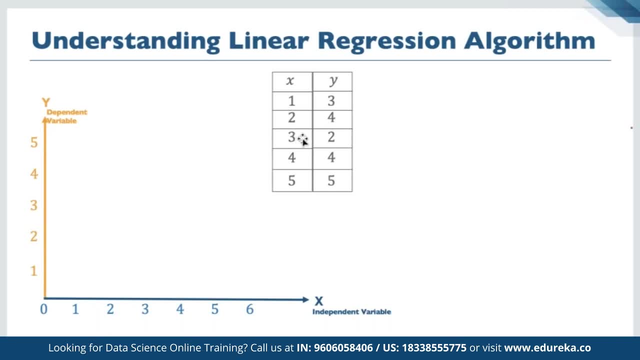 when X is 2, value of 4, when 3 values 2, when 4 values 4 and then 5 values 5.. So these are some point that we have to draw. So in the graph we draw that point: X versus Y. 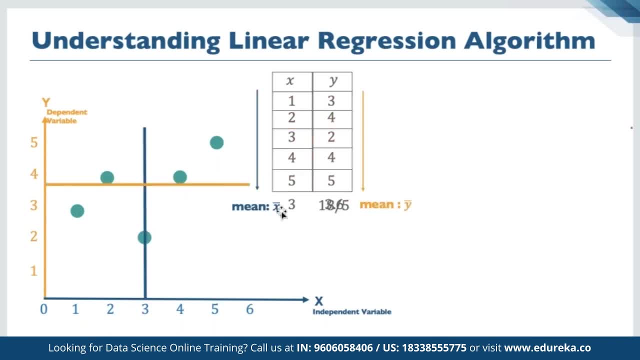 Now, after drawing that point So we can, we have to calculate the value of slope, because there is a value of slope, Then we know which is the best fit point. First of all to calculate that value of. take a mean of, that means means, sum of all divided. 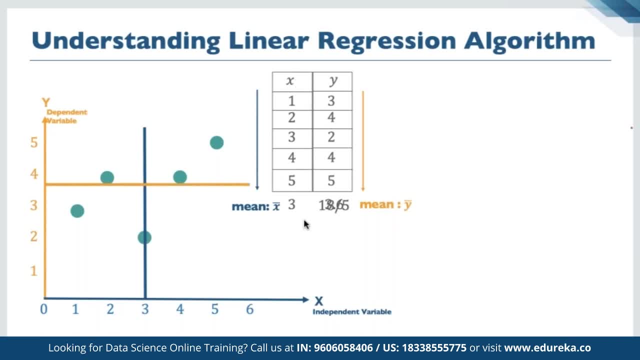 by total number of value. total value divided by. divided by number of values, like will calculate all of them divided by 5: mean of X and mean of Y. The formula for that is: when we get to the mean of X and mean of Y know we find out that 3.3 versus 3.6 is one. 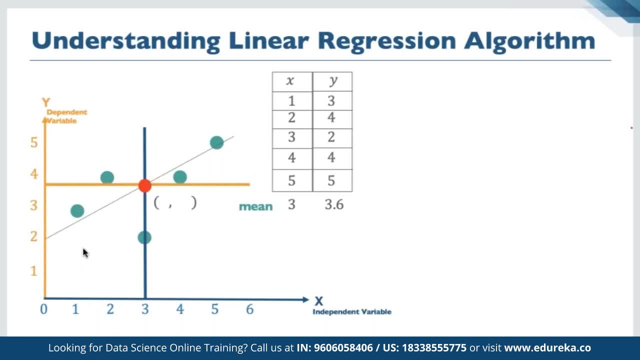 of my best point because the best fit point. now we draw one straight line from there, We'll draw one straight line from this point, like this XS. Then we figure out that what is a point that like on this particular line and the point that lie? 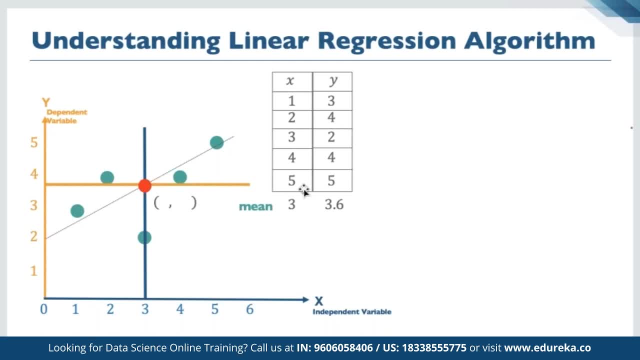 over. this line is the best. fit line means if we say it's a completely dependent. if the price increase by 5 or the price decrease by 5, the sale increase by 5 is more like that. Now we carry the value of M how to the value of M. 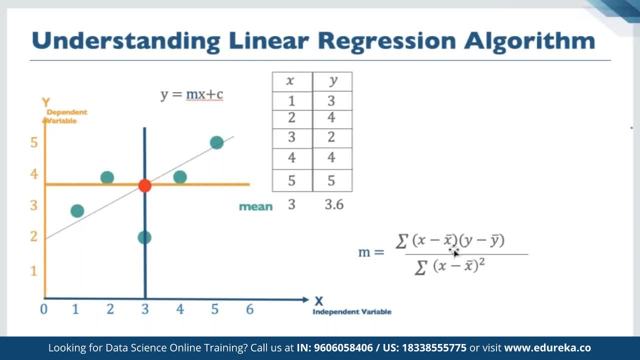 So it's a epsilon of X minus mean of X, multiplied by Y minus mean of Y, divided by X minus mean of X square. This will help you to tell the value of M, X minus mean of X, Like the cervical, the X mean of X, Y minus mean. 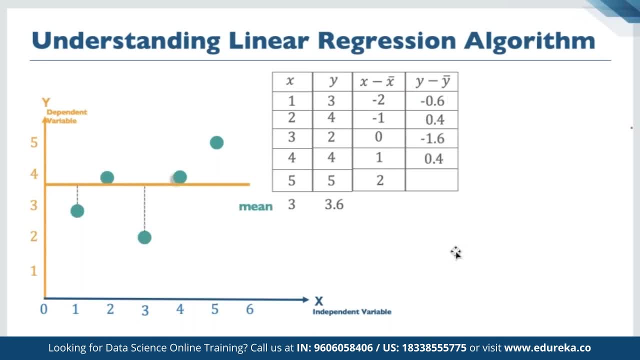 of Y. we calculate Now X minus mean of X square And then We'll do the multiplication of them And at the end we find out that X minus X, Y, X square is 10 is 4. divided by 10 means 0.4.. 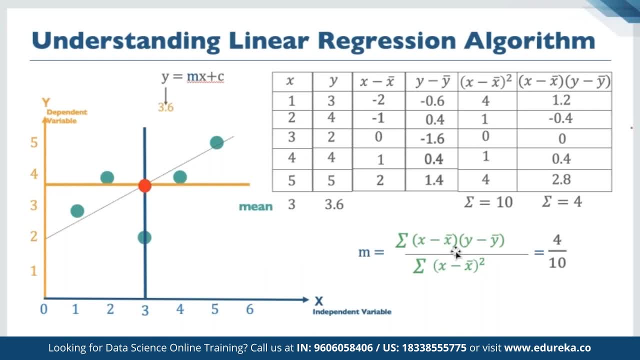 The value come out to be 0.4.. So now your value of Y is 3.6, value of X is 3, value of M is 0.4.. Now we can tell you the value of C. Now C will be your 2.4.. 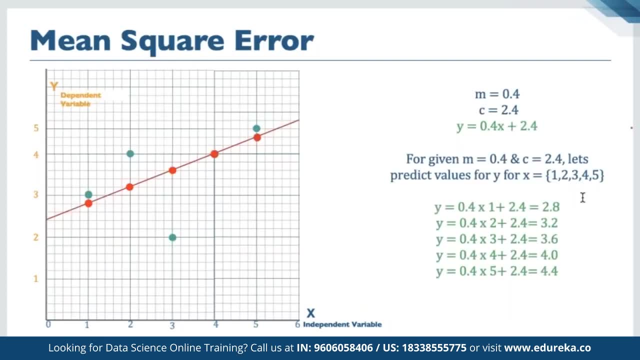 C will be your 2.4.. So now, on the basis of the 2.4, for given value of M, the C is 2.4.. Let's pick the value of M 1, 2, 3 for now. So how we draw the slope now. 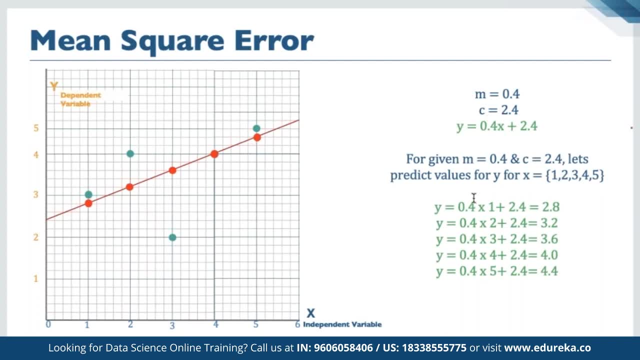 we know the value of C, How we draw the slope. value of X is 1.. So Y is equal to 0.4 x 1 plus 2.4. 2.8 means when a value of X is 1, Y will be 2.8. 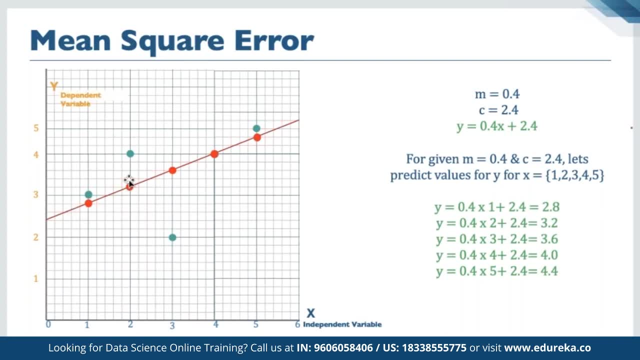 when value of X is 2, value will be 3.2. when values 2.4, values 3.6. like that way, I take out all the five point and draw one straight line, because I get the value, all the value I'm able to find out. 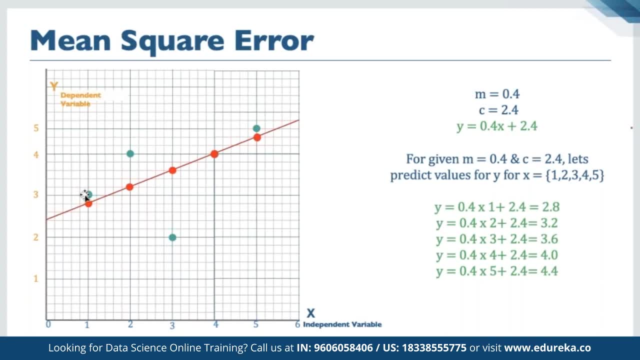 and I have drawn one straight line there and now. what all points lies near the state point, if particular the one that's our best fit model, when it say that when the price of that will be one, the sale is three, and when the price of that is five, the sale is. 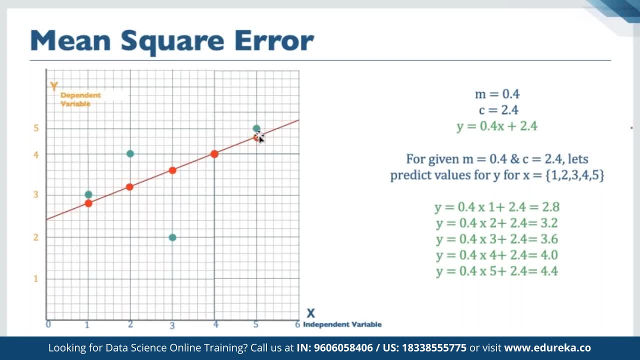 around five point something, four point something. So this will figure out that how exactly your best fit line can be drawn and for drawing that, this is a formula that we calculated. Now, that's a regression line that we able to draw, not distance between the extra predicted value. 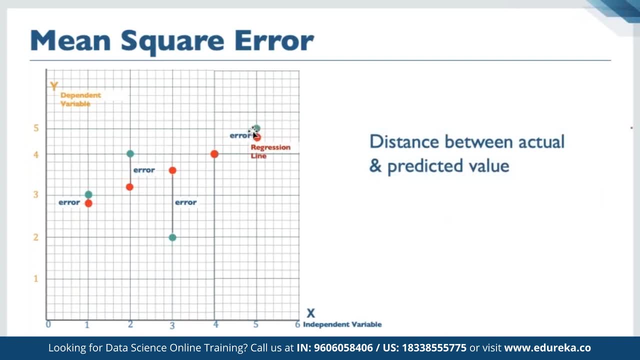 What is the actual value was a predicted value. Now we calculate distance between them and according to the distance, you will come to know that what is the right fit value that you should take means what- how exactly you should play with your model in terms of a best fit criteria. 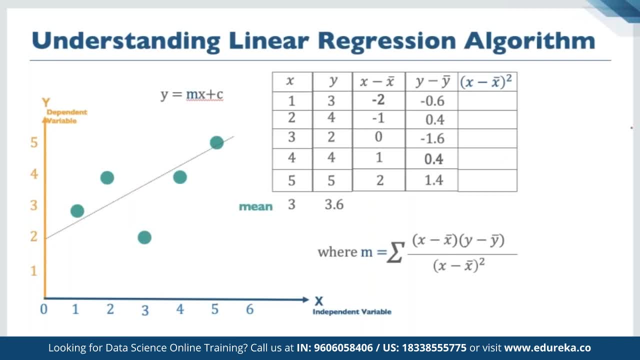 Now you have given some values like this: Initially, you wish you have been the value like this. Now you have drawn some point according to that. Now you will design the best fit line. for designing the best fit line, What to do is you have to first of all calculate the value of M. 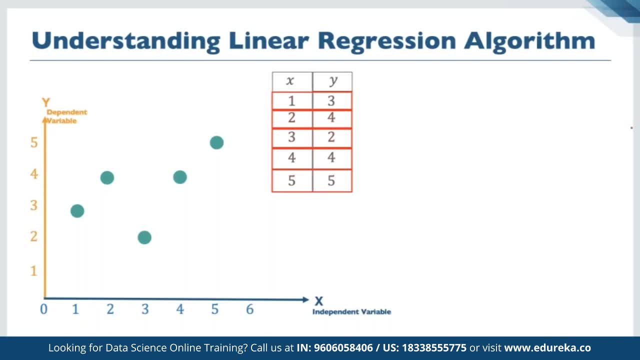 And if I say the value of M now, to give a value of M in a formula, is X minus mean of X, Y minus mean of Y, divided by X minus mean of X, square, whole square, We can get X minus mean of X. then we keep on calculating that. 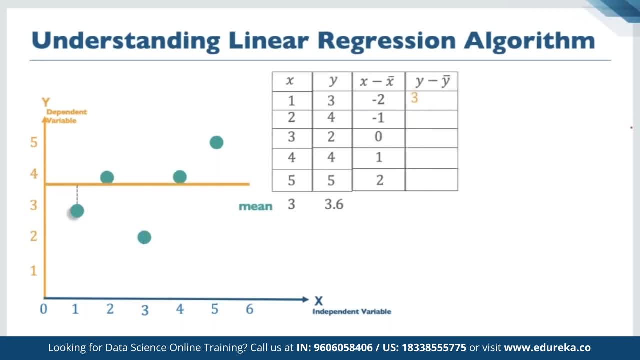 and then we start killing Y, Y minus mean of Y. Now, once we get the value of Y also, the formula is: X minus mean of X, multiply Y minus mean of Y divided by X minus mean of X, square. Now I take the value of this and the square root. 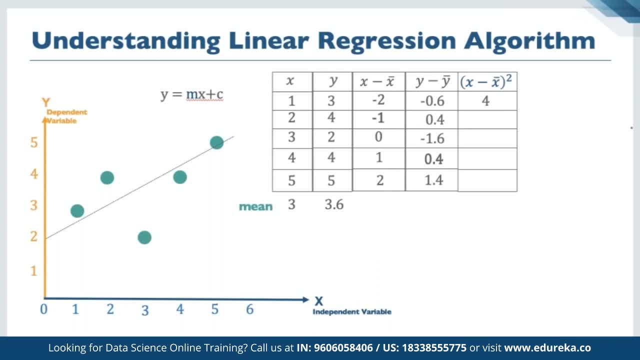 of that value is about 2 of that value. So then we get this values. Now, ultimately, the last thing we have to calculate is Y minus X, minus the mean of X, multiplied by Y minus mean of Y. So we calculated that value also. 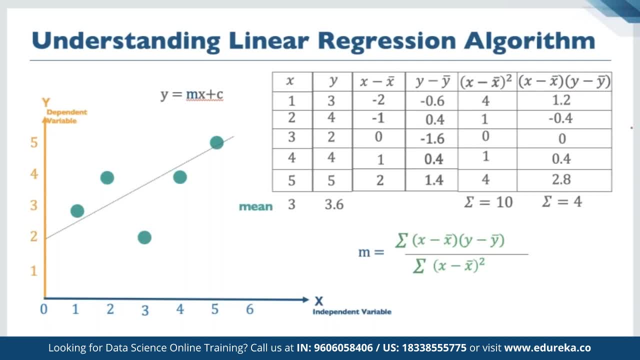 Now, once you are able to calculate this value also, Now we start putting that into our formula. Our formula say that 4 divided by 10.. So we get one value of M. M is a middle value- We get 0.4.. 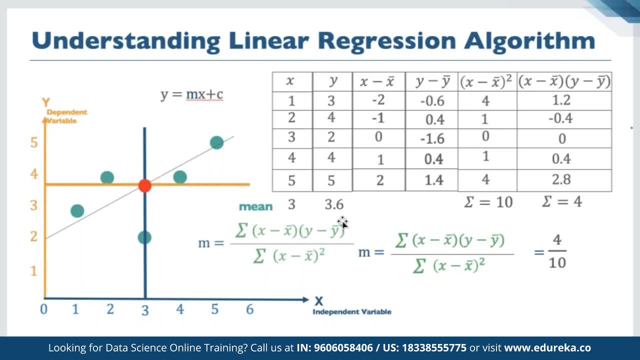 So we draw that X minus mean of X, So 3 for value of the x-axis and 3.6 on y-axis. This is, although, my main point, So this is my center point now across, that when I start writing the value of, I now value of M also, X also, Y also. 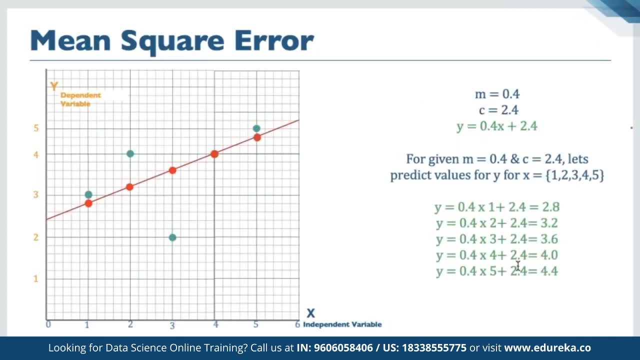 So we can start taking the value of C Once we tell the value of C. Y is equal to MX plus C, So value of X is there. What should the value of Y with respect to X means? What is the value of an independent variable? 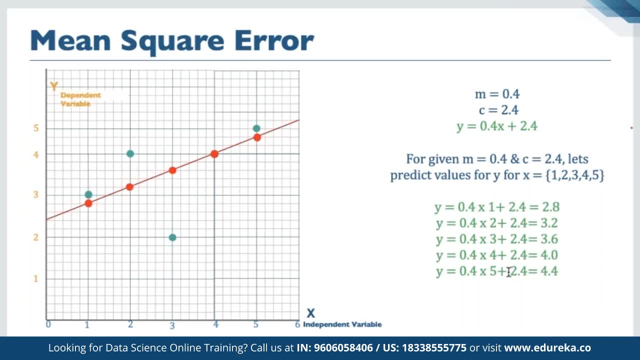 with respect to dependent variable. So we'll tell like this will say: when the value of X is 1, Y is 2.8. when value of X is 2, Y is 3.2, 3.6, 4 and 4.4.. 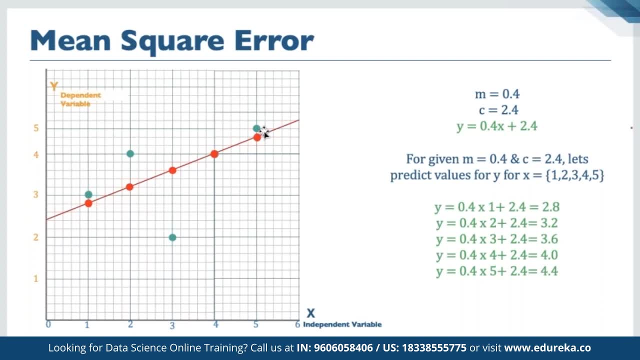 So we take all these points and draw one straight line and then, with the all, all the point that we initially map, Now we check that which answer is correct, So we find out that the first and the first and the last one is the right prediction. 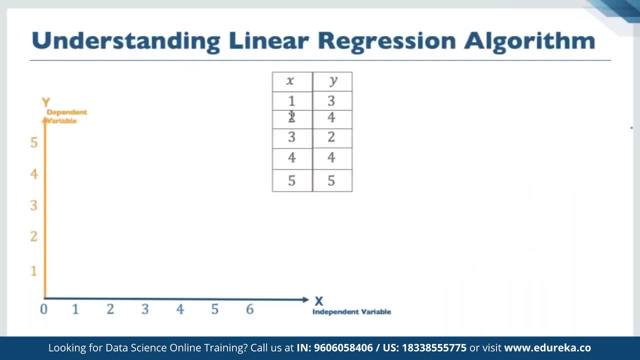 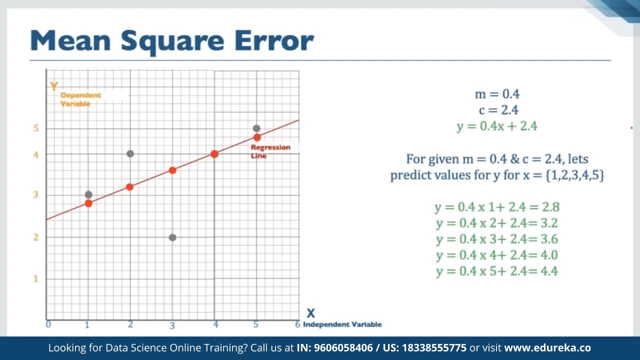 so that we should follow: X was 1 and Y is 3 and a value of 5 versus 5 means it say that how exactly they are dependent to each other. that you calculate on the linear regression. I try to draw a letter, one code for you guys. 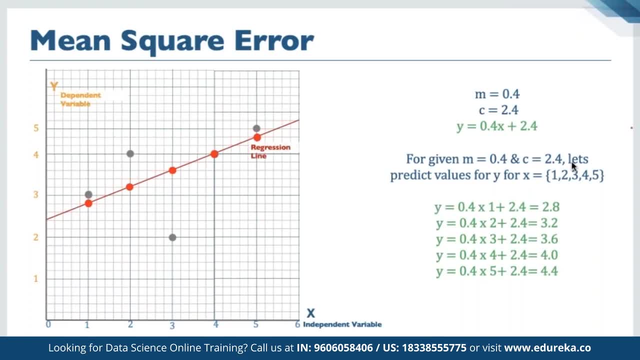 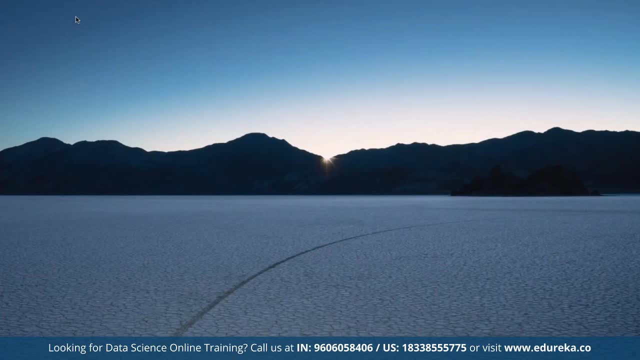 Also that you more understanding. Now for doing that linear regression: Generally, we pick our code editor and we can go with the co-editor of anaconda And we are going to the Jupiter notebook to write our code. First of all, I have some data set with me. 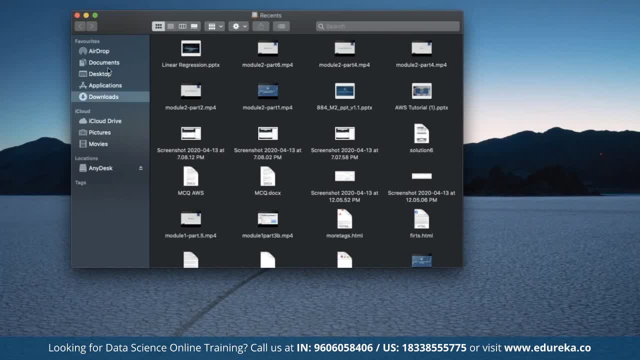 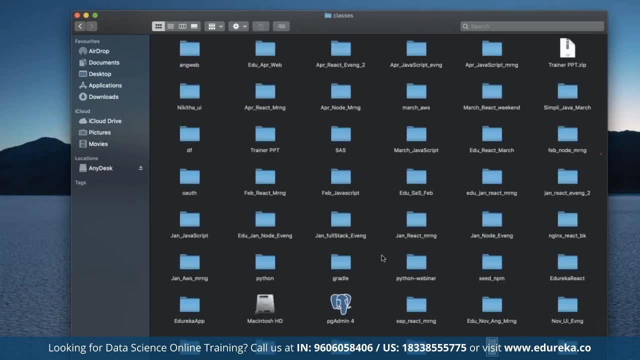 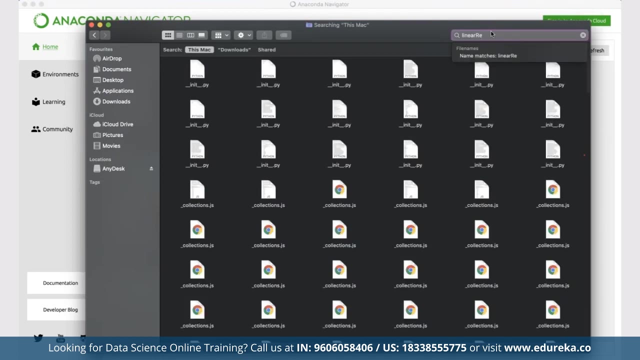 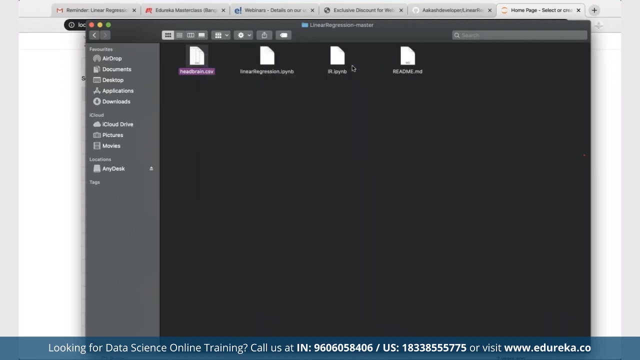 Let me get that data. You can predict over any data set. Let me see that code is here or not. Else, I'll just download the data set. basically, Now, guys, we have one data for the head brains. Let's first see this data set. 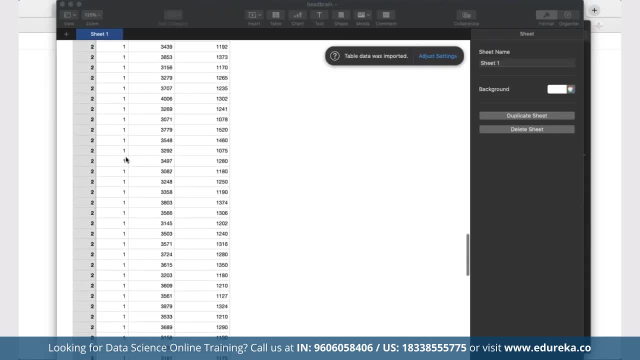 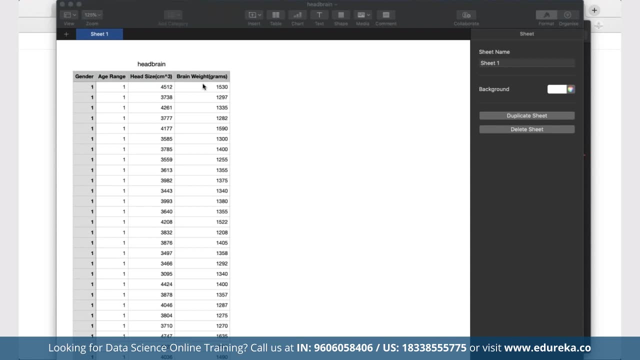 I say that the age- and we have head size and a brain weight- means according to the head size of a person, How much will be the brain weight? I want to predict that. I want to get a best fit prediction Now for doing that thing. 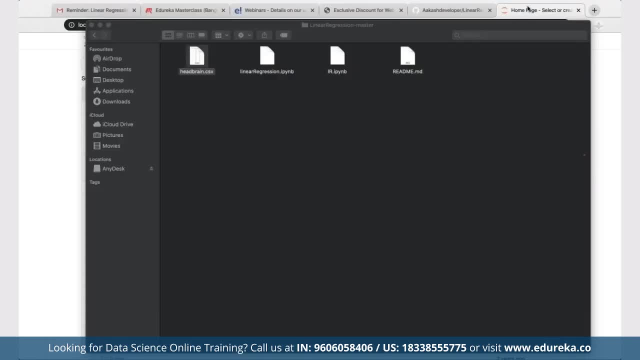 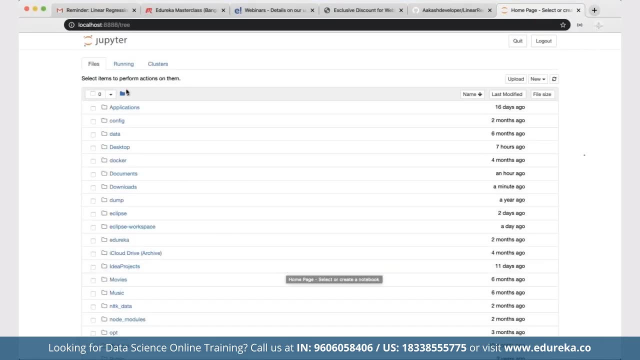 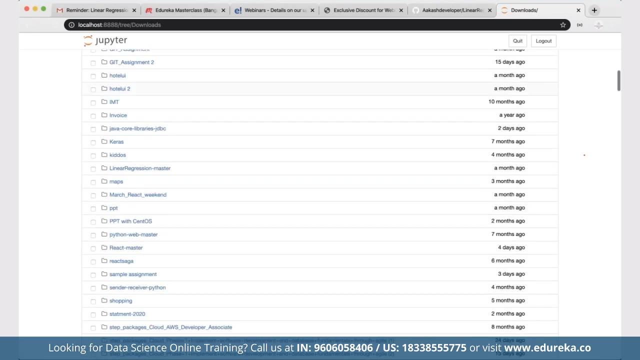 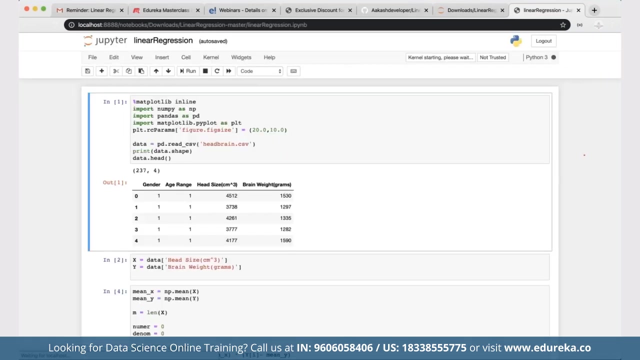 So we use this data, fossil CSV data We already have. now I'll open our, which I'll go to the downloads There. I pick this linear regression Here I have: the Jupiter notebook is now in this Jupiter notebook. The very first thing is how to play with that. 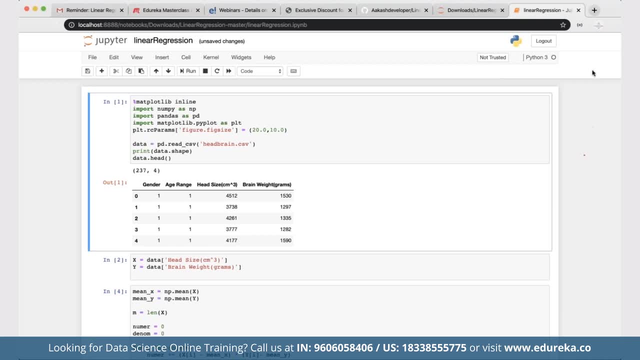 I'm going to draw the graph. I'm to draw that graph. We have to use a matplotlib Over that matplotlib. I'm going to draw that graph How. first of all, I use a matplotlib here. Then I import numpy. numpy is basically. 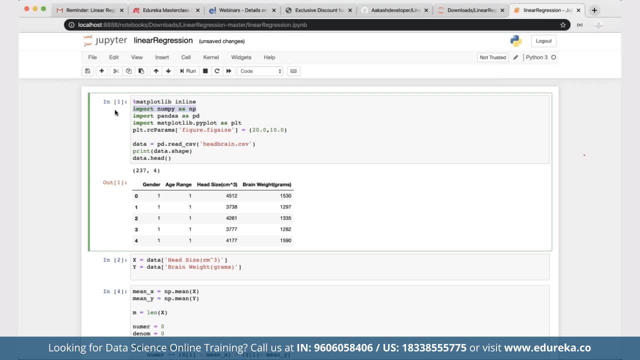 to make the things into array, We use numpy. numpy will give us the array, the tensor kind of a graph array that I have to play with pandas. pandas is basically to figure out the model to do the calculation. We use pandas and matplotlib to draw that graph. 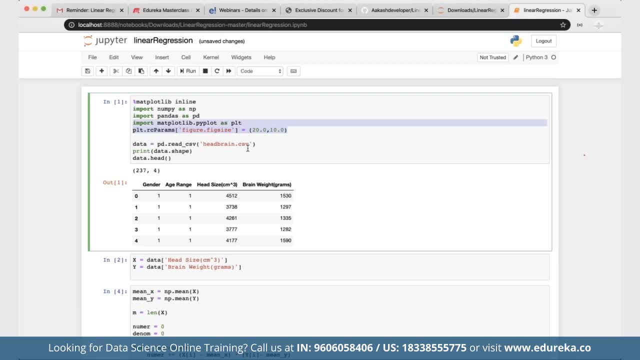 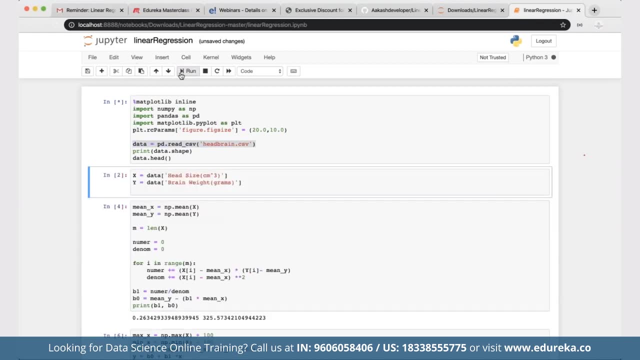 Now we give the figure size for a matplotlib. Now data We are reading from the head brains CSV file. We can just run this first step and we come to know: Are we able to get the data or not In my own account. 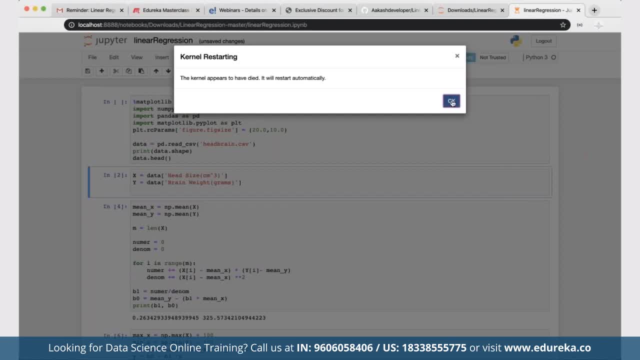 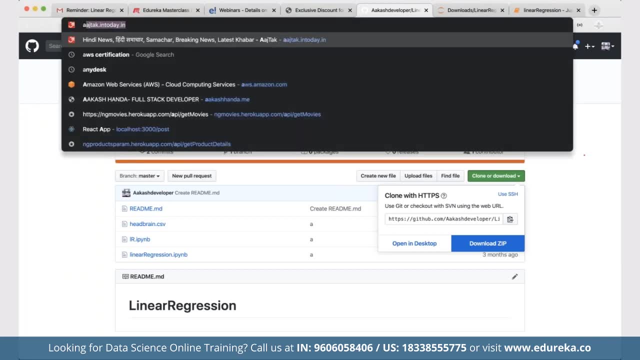 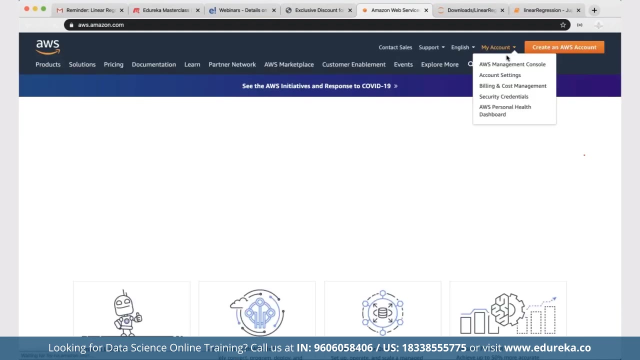 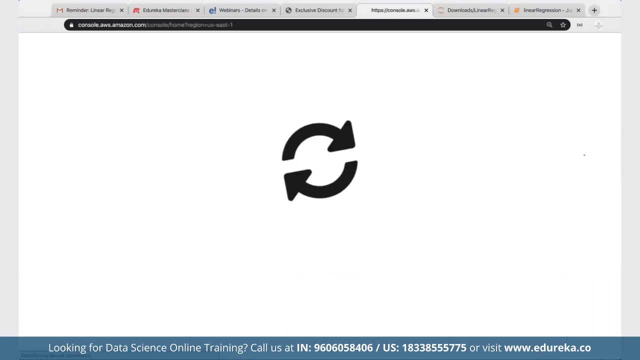 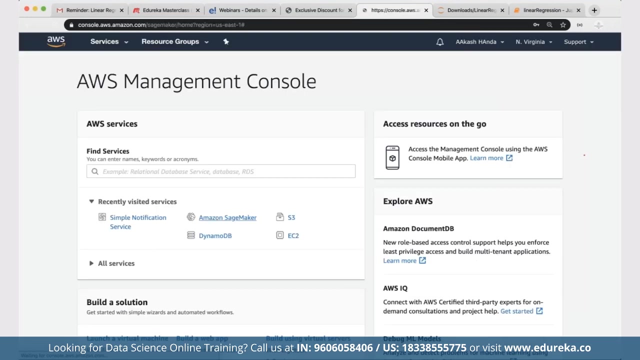 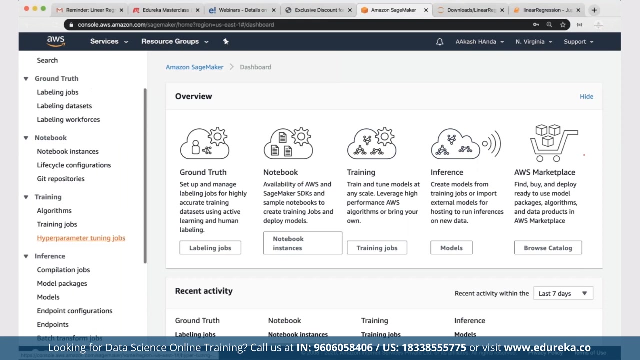 I'm getting one issue. I'll do one thing: I'll run it over the Sage maker. I'll do one thing, I'll run it over the Sage maker: I'll a Jupiter notebook over the cloud. Now, now, from here, I'll launch my notebook instance. 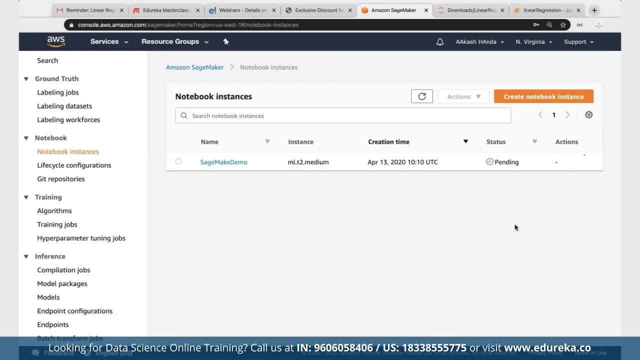 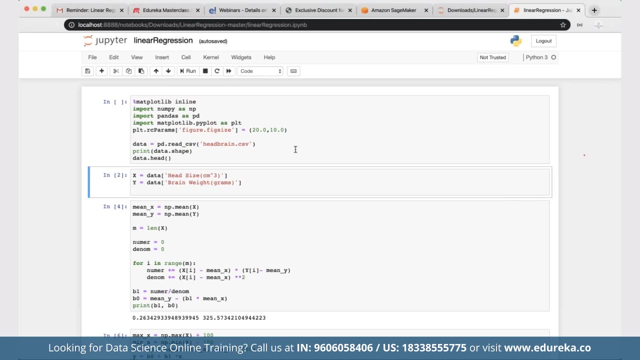 After started. it take a few minutes to start that. while it's starting now, I'll explain you the code. once it started properly will run that Jupiter notebook here and we test that. Use a matplotlib. Then what it do is always open one small square window. 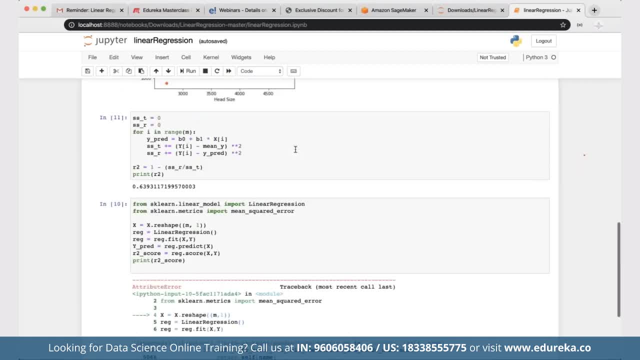 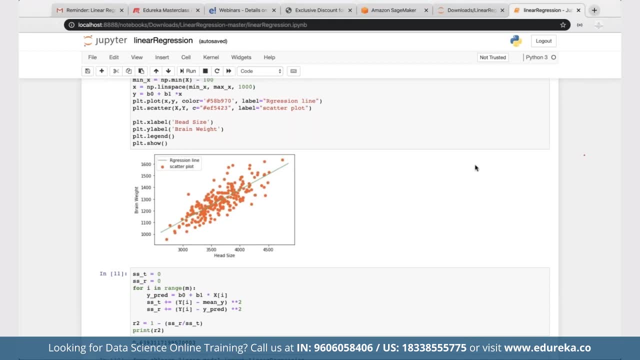 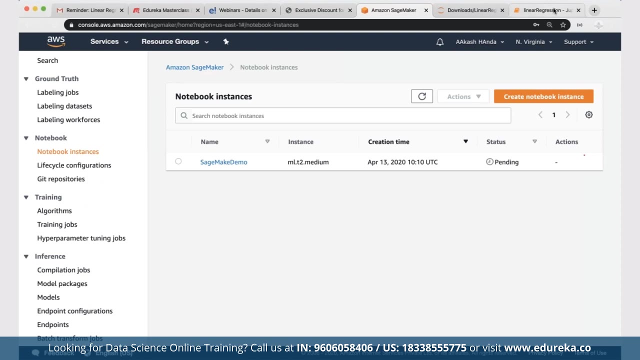 in that that graphs are visible, But with this, the graph is directly visible here itself. like this: You have another window. we show the graph here itself. Now, guys, while my notebook is running, Starting as of now, Let's understand this code. Now, here we have two variable: 1x, 1y. 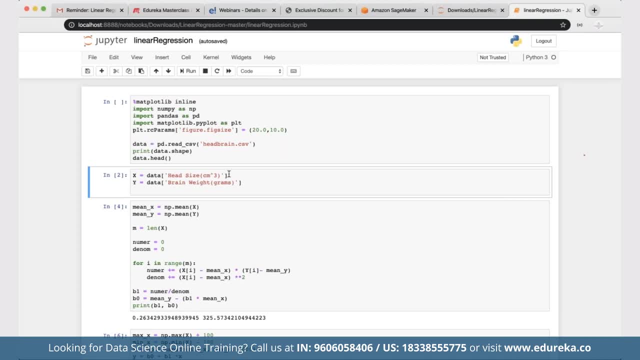 So X is the head size and Y is a brain weight. Now we remember the formula: X minus mean of X multiplied by Y, minus mean of Y divided by X minus mean of X whole square. with that formula We catch the value of M. 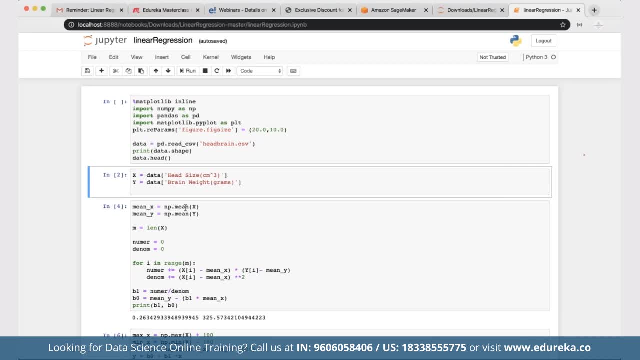 So we'll say for some mean of X numpy dot, mean of X numpy, mean of Y and M is equal to length of X, that M is a length of X mean. And then I'll take one numerator and denominator, 0, 0. Now what I'll do is I can find the value of numerator. 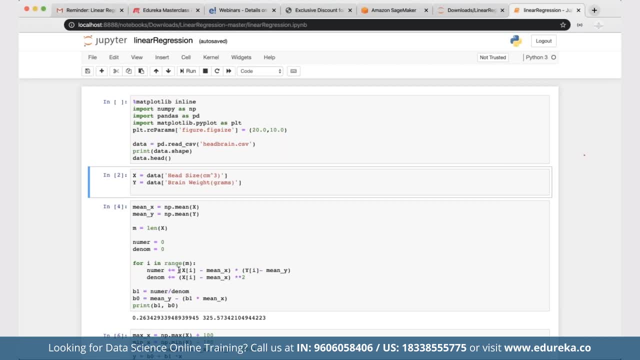 and denominator. So numerator will be X minus mean of X, multiplied by Y minus mean of Y, and denominator is X minus mean of X, whole square. Now when I calculate the value of D, 1 is numerator versus denominator means. I'll get the value of M here. now Y is equal to mean of Y. 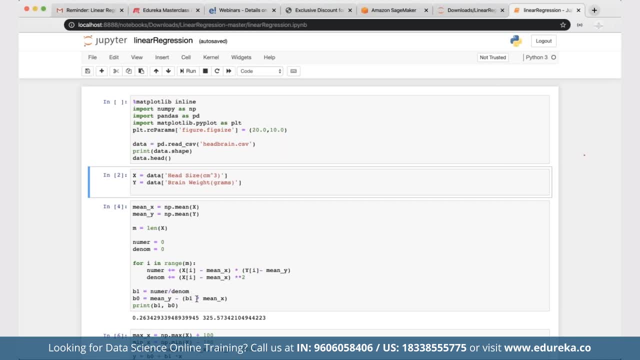 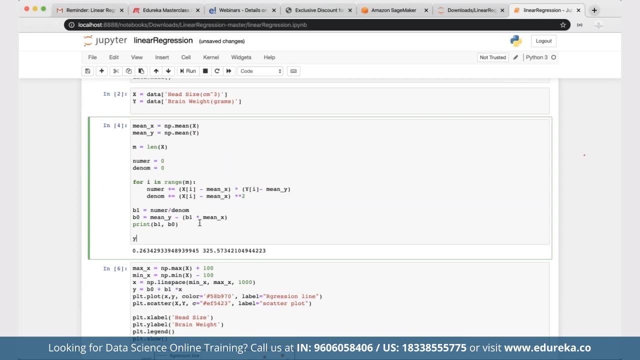 Minus B, 1, that is your M multiplied by X. What the formula? the formula is? Y is equal to MX plus C. What they're doing here is: we have the value of Y. Now we have to tell you the value of C. 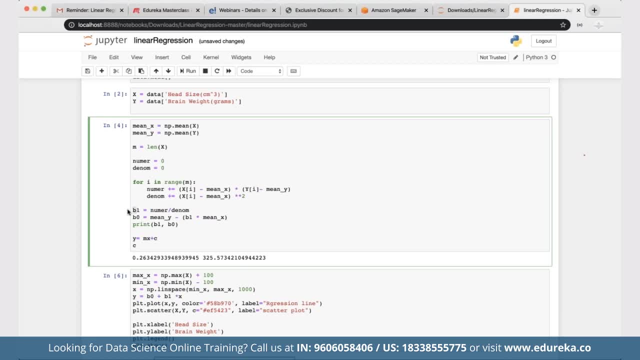 Correct to tell. the value of C, B 1 is equal to equal, equivalent to your M. So what color value of C will be? Y minus M, X? right here. Why is mean of Y minus M? you already calculate. multiply by X, you will buy this. you will get the value of C. 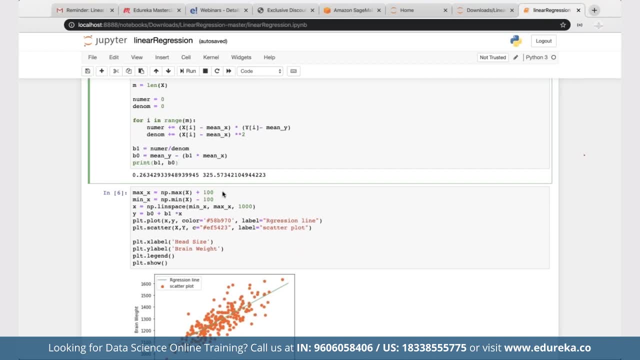 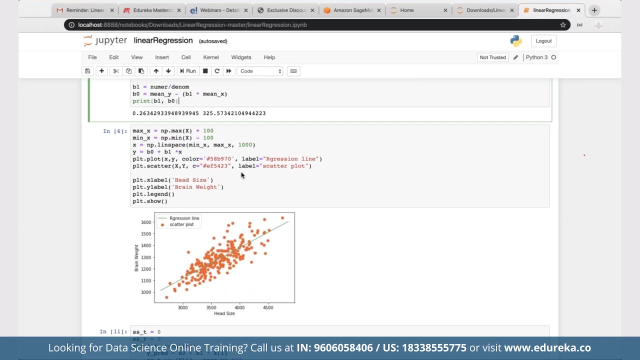 Now, after that, now our numpy array will do plus 100 with that and minus 100 with that. now will say NP, dot line, space, X, Y and thousand. now we draw that plot. We draw that plot by the, using a formula, The main line. 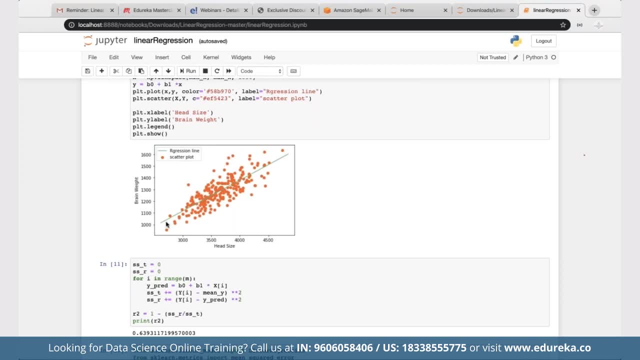 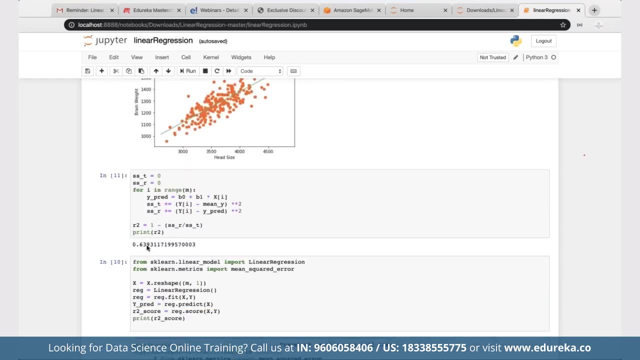 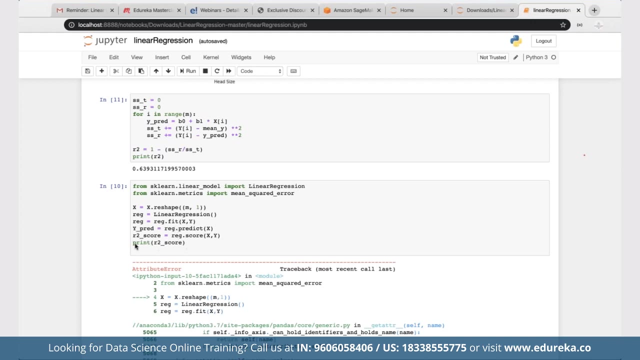 and then we'll draw the plot of. that is all the values that we have. these are main line here. Now we will predict the value of the mean- the mean is 6.39- and then with a Skyline model of linear regression, We will actually figure out what is the predicted value. 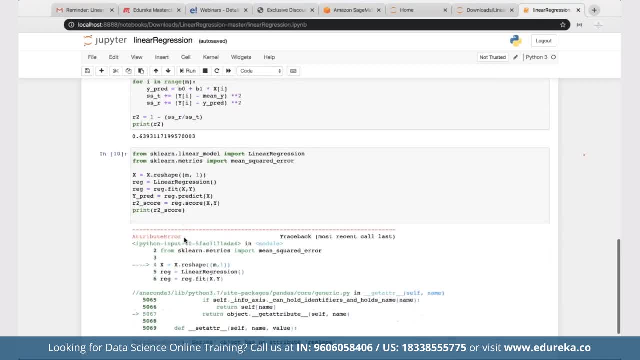 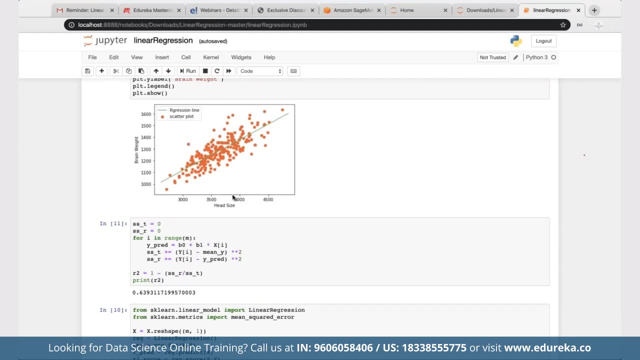 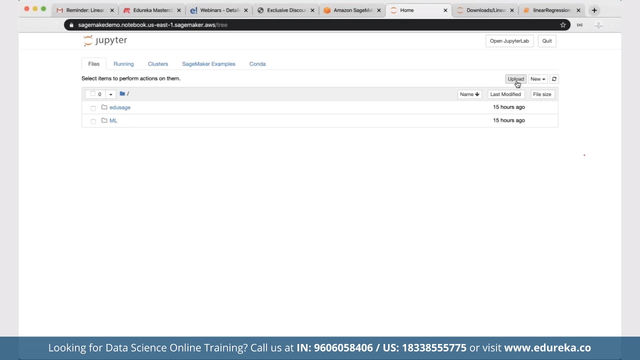 What the predicted score and there will calculate that, Okay, This is the best fit Score. that where the head size is, this brain size will be this. So now we do all our calculation over that values. So let me just upload one folder here. 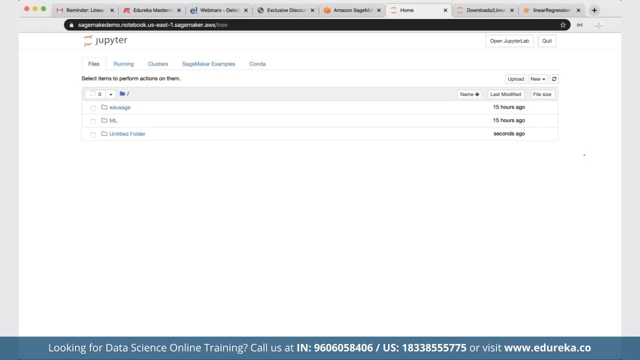 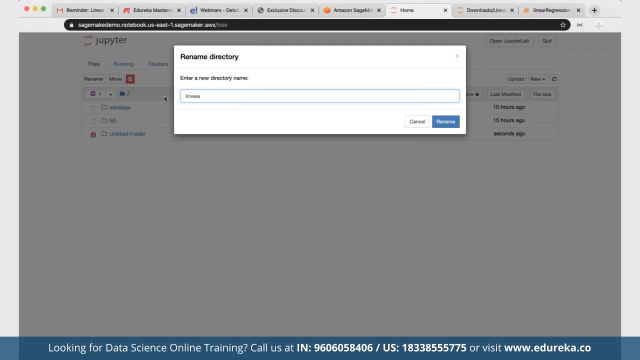 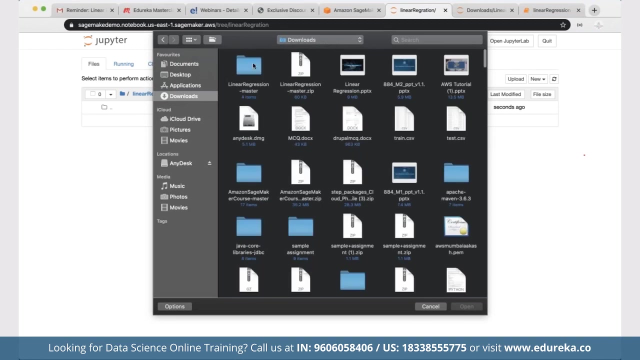 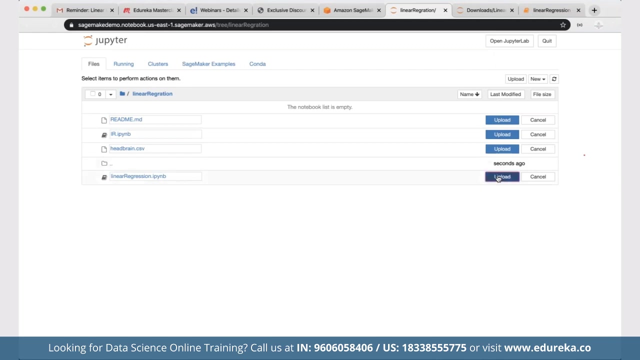 And with a new folder here. first of all, One second. Let me rename this folder. We'll tell you in your regression Now. in this I'll upload all the files Now, notes, in a regression Now. after that we'll open a notebook. 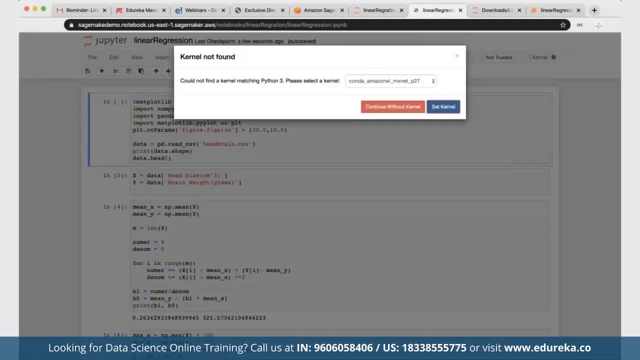 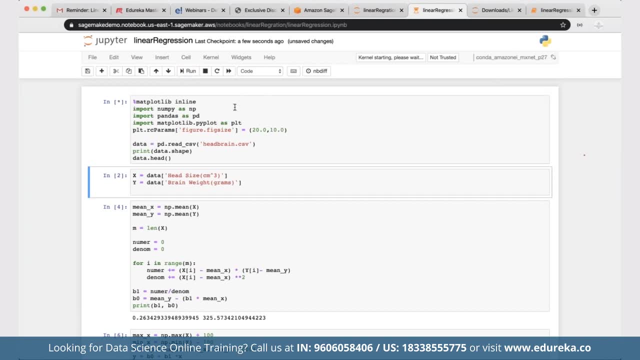 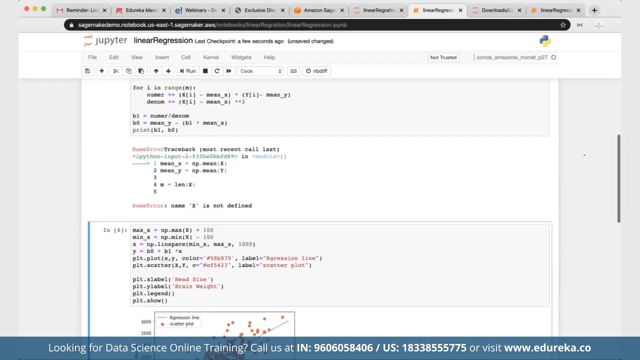 Let's try to run that. We'll set the current value Now. this is the first point we able to read our will, be able to read our data. Then we'll set the value of X and value of Y. Then we actually take out the value. 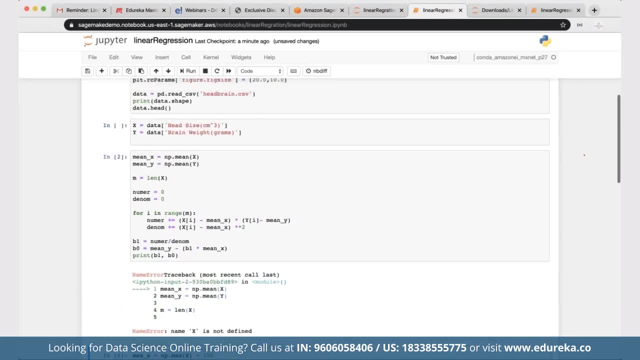 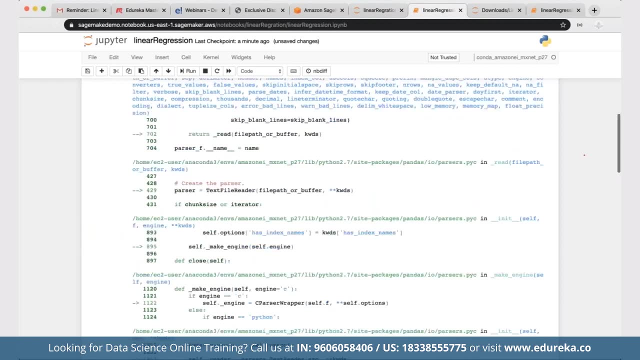 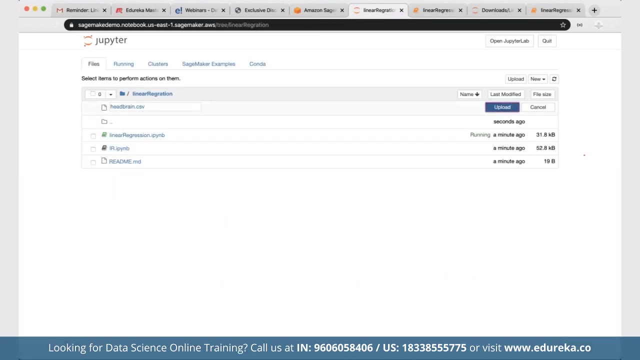 It's a X is not defined. Once again, When we run this piece of a code, The file does not exist, Although we uploaded that file. just verify once: Oh, that file is there always, or not uploaded. That's why, fine, Now run once again. 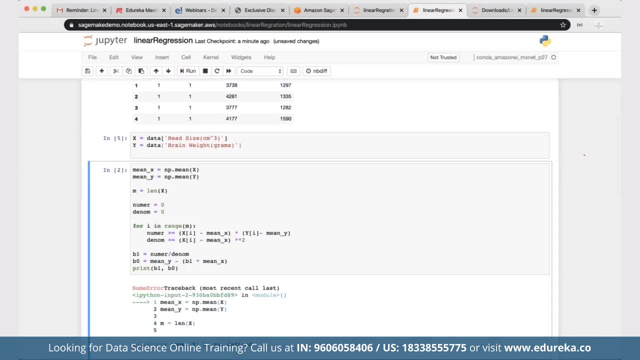 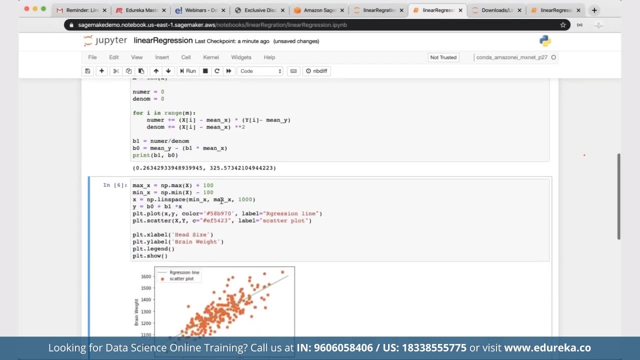 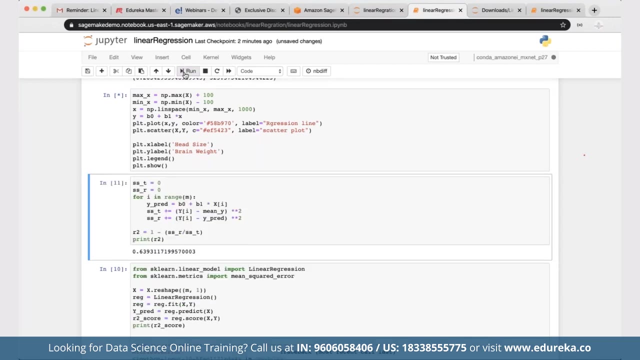 Yeah, now you will read that file. here We'll define X and Y variable. Now we calculate the value of M and we plot- see- the value of M and C. on the basis of that, we plot one graph for us. This see the state line and is a point near to that. 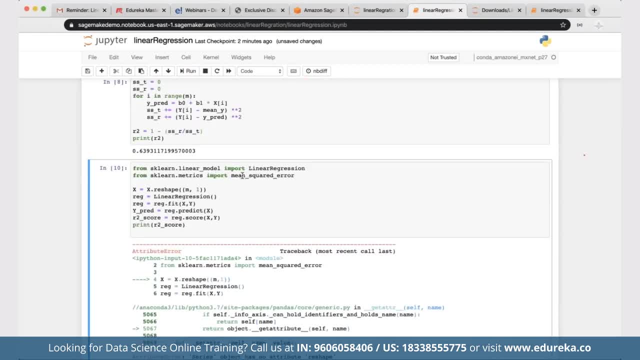 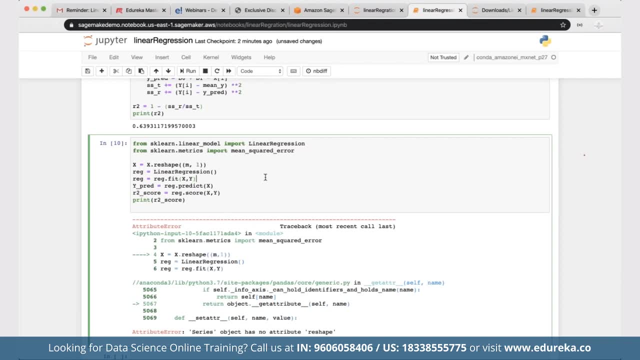 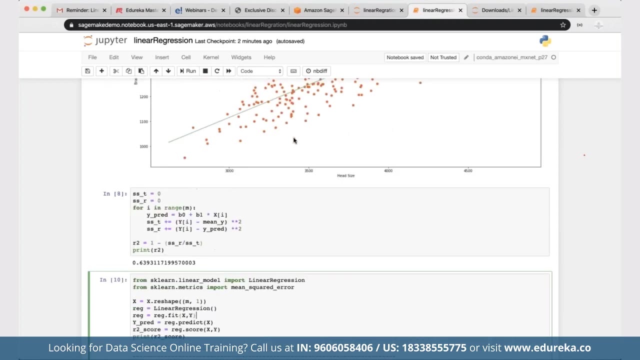 and then we'll figure out a best State value for us. There's some variable issue. Any variable is not defined properly, Let's say a series object, So here we get that predicted value. Now I'm trying to achieve the same thing with the Skyline. 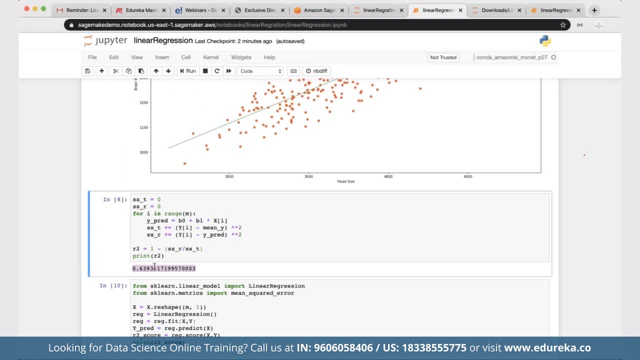 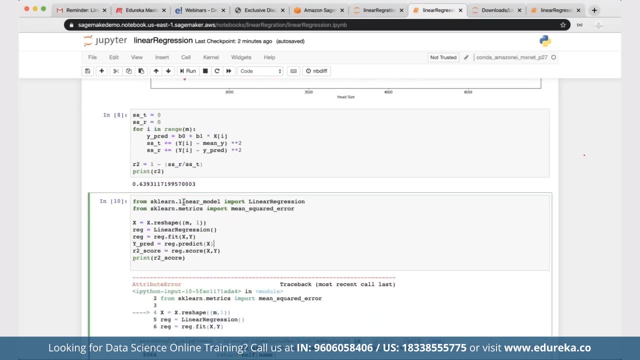 So basically, till this point, your things are done. You came to know what is the actual value, that you have to work on how fit your model is. now I'm trying to a same thing with the Skyline also. This is something you write- everything manually. 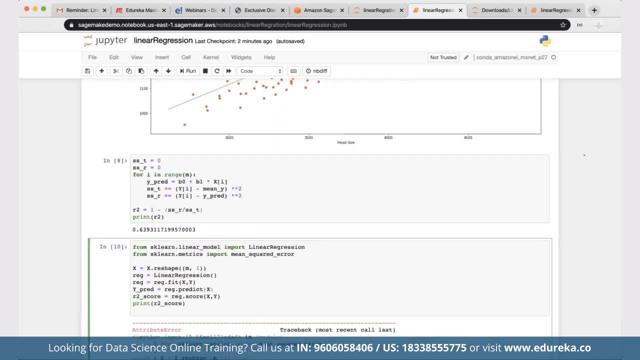 by Panda and numpy. You can achieve that, these value with a Skyline model, as my Skyline model is something that they give us a directly. They have already built algorithm. What we have to do is we just have to start to use that algorithm directly. 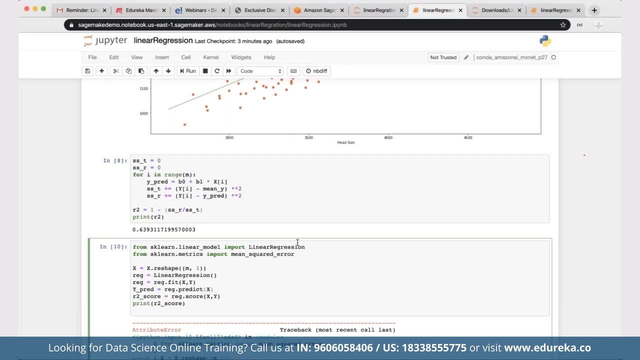 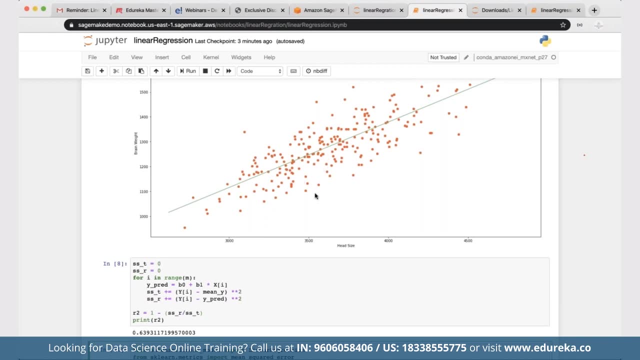 So that's where we are finding some more things that I can check that relatively from here We find out the best fit value is 6.39.. So 60: 63%. that model is accurate. and now we have find the middle value also. 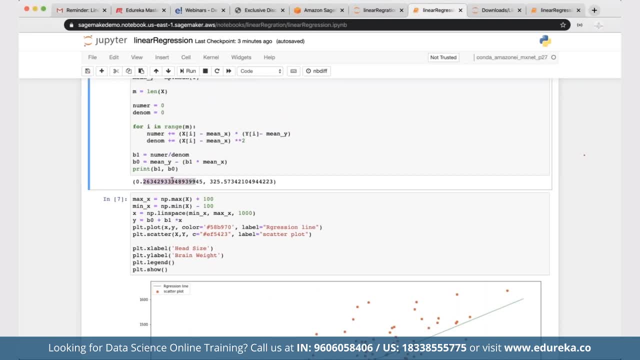 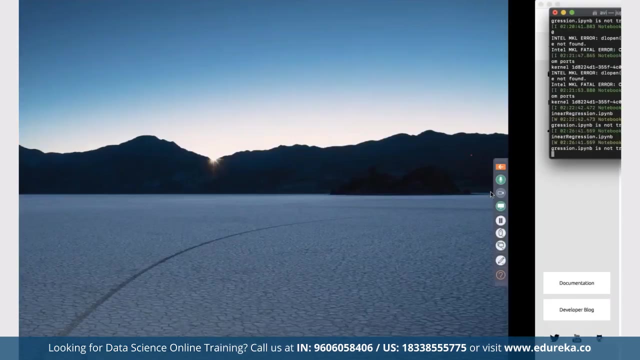 when the size a headband is like this: This is a size or this is a weight, this actual value. now, over this I can do my own prediction. So, basically, we just calculated that value and you plot that on the graph. So this is what we want to achieve to linear regression. 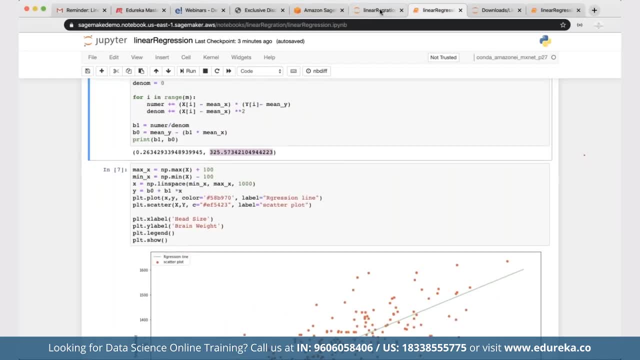 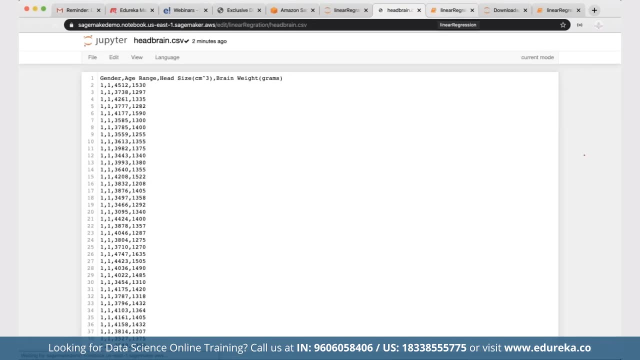 that how independent and dependent variable behave. Now we go back and check our headband CSV. Now exactly it look like. let's see It say that when the head size is this, the brain size is this. so now we able to calculate that about the best fit model. 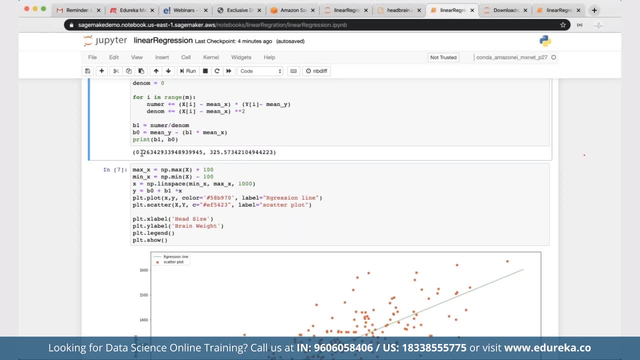 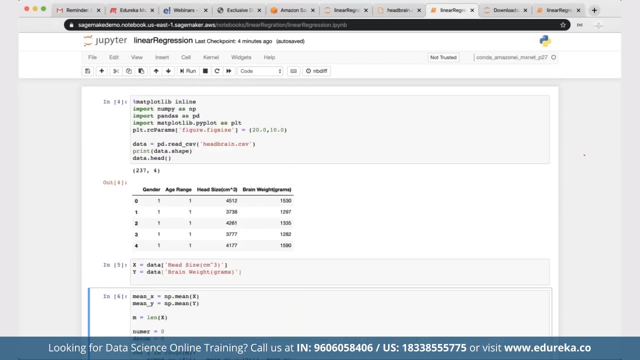 when they, when the head size is this, the weight will be this. now do all the calculation over this. That is how, guys, you do your linear regression model. It's a core is the most simplest form of the machine learning learning algorithm from where you can do the prediction. 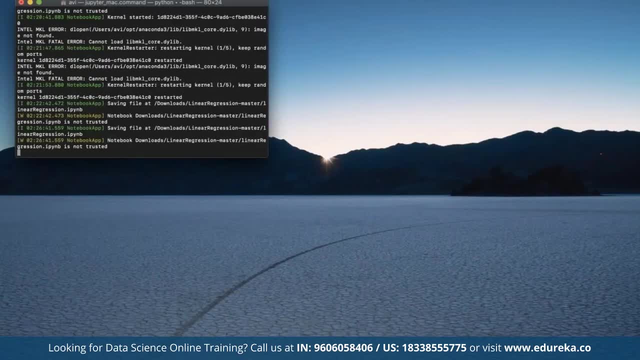 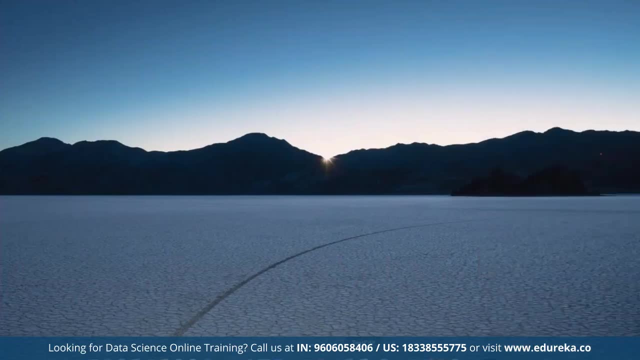 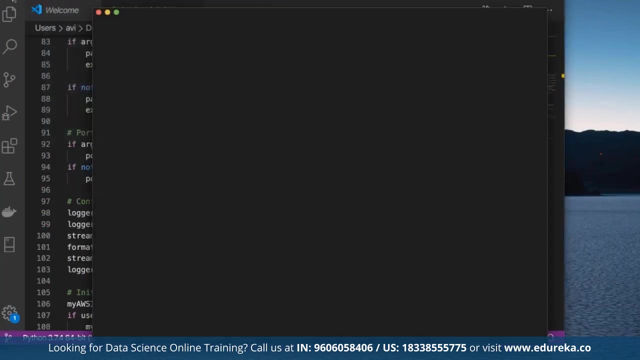 And to run the code a two-way either. download the anaconda. with anaconda you get the Jupiter notebook. You can run that, Although nowadays we have visual studio code. this visual studio code also give us an option to run our notebook In my system as a some kernel issue. that's only point. 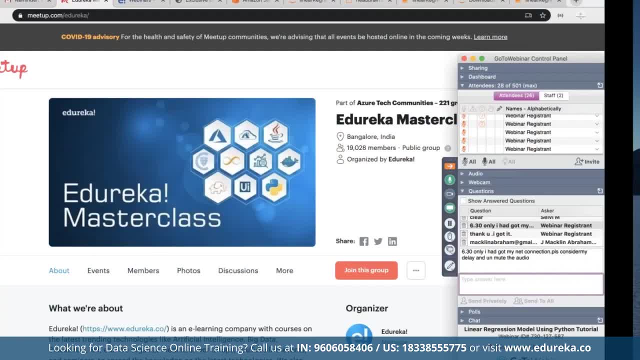 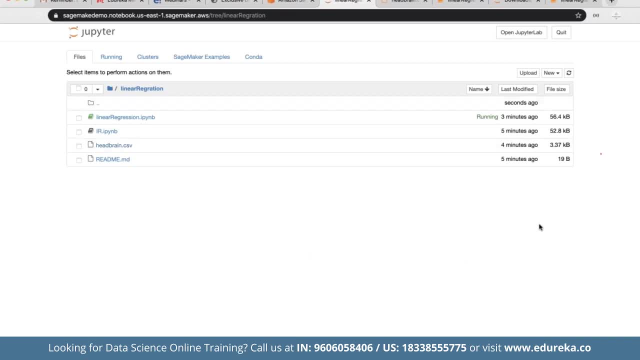 So I prefer to run it over the cloud. the benefit of running over the cloud is that it is I don't have to take care of any other thing. My cloud will take care of each and everything there. So that's why I prefer to run that things on the cloud. 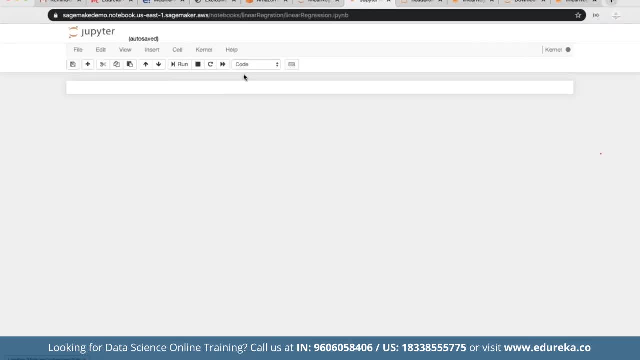 and do that because it gave me some more modeling. also because I'm doing some more algorithm over that. I have a lot of ml stuff which actually I'm working over that and all the things are on my ml enrollment. Cool is I think they are done for a session. 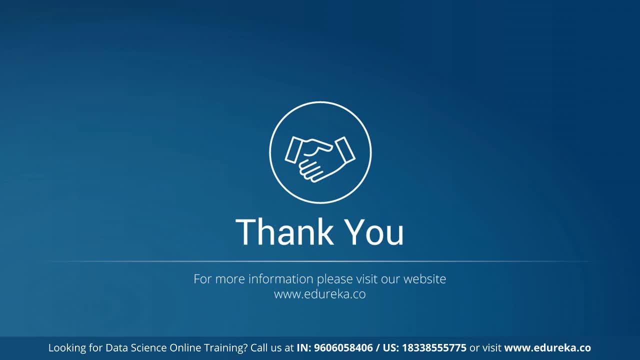 Thanks a lot for joining. Bye, Bye. Take care, Stay at home, Take care of you and your family. Thank you, Bye, Bye, Bye, Bye. 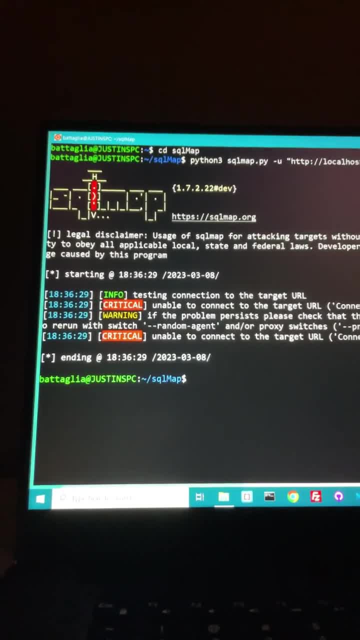 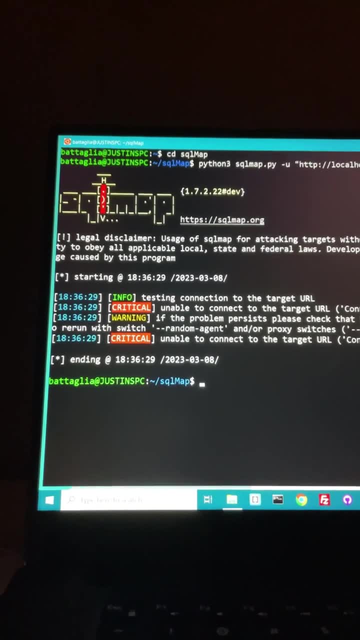 Yo, what's up, guys? It's Big Code Hours. Put out a poll and it looks like you guys wanted me to try to hack into the bank again, so we're going to do that. I'm going to try to use SQL Map, We're going to upgrade the security and we're going to see if we can get in there.